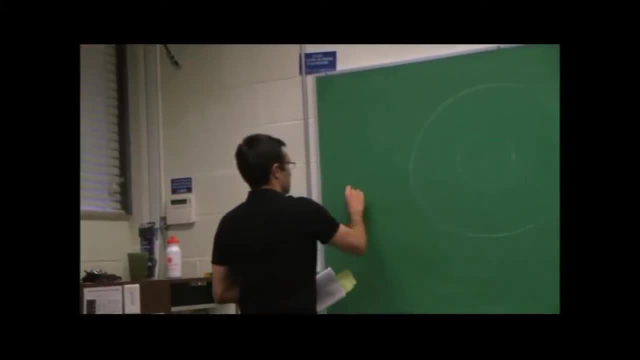 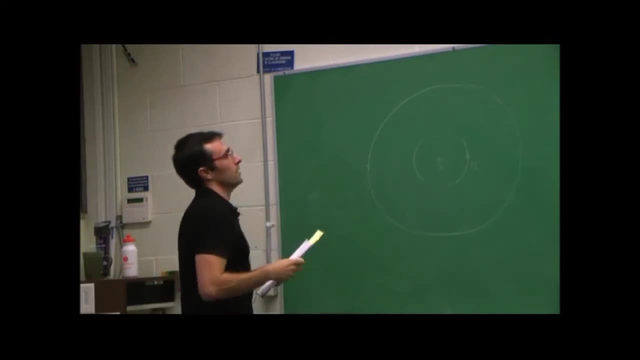 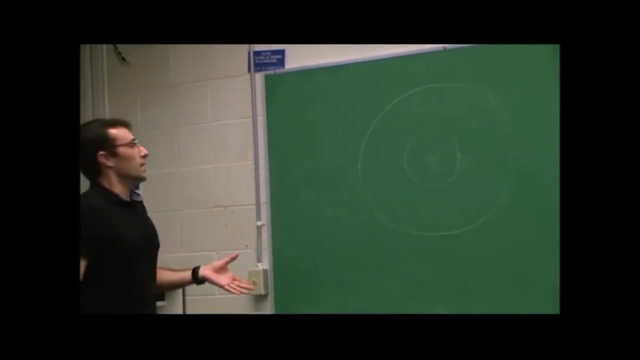 So we use what we call the patched conics method, which means you're patching conics Inside the sphere of influence of planet one. you don't see anything else, so you do everything that we have done so far. Of course, you want to leave that. Which means you have to go on a hyperbolic path that eventually will lead you outside of this imaginary sphere of influence. and once you are outside of that, you're just going on this Hohmann transfer and you invert the transition once you get to planet two. 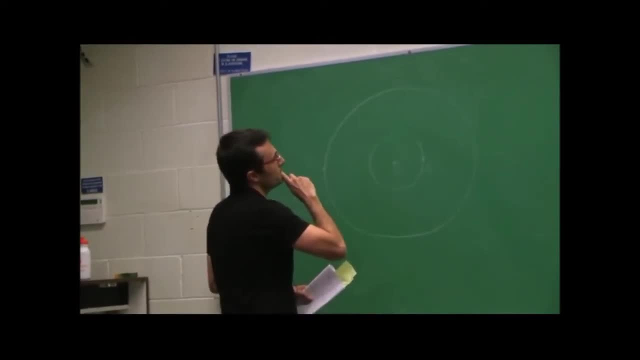 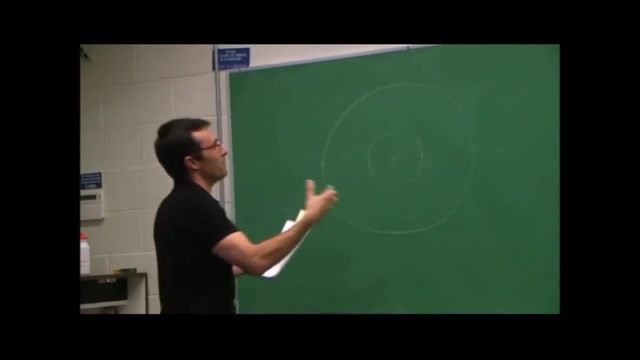 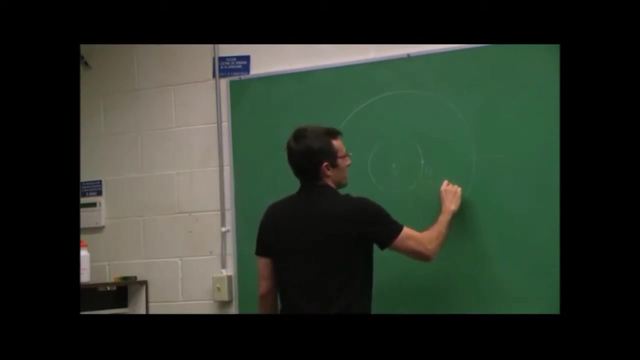 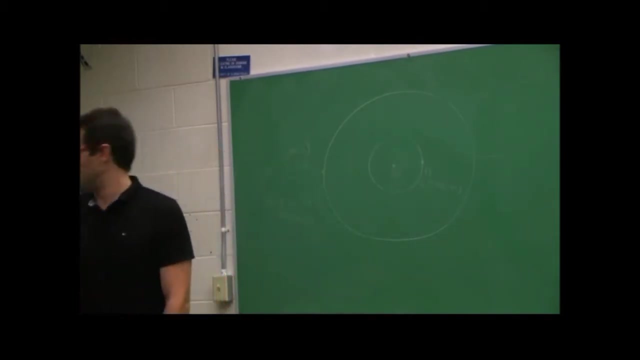 So the video that I gave you should have stopped at the point of basically doing this computing. you know timing these maneuvers. If we're doing a two-impulse burn and let's assume that once and for all, this is Earth and maybe this is Mars, because everybody's talking about these days- and that's most of the problems that you have on your book- Mars and Earth- 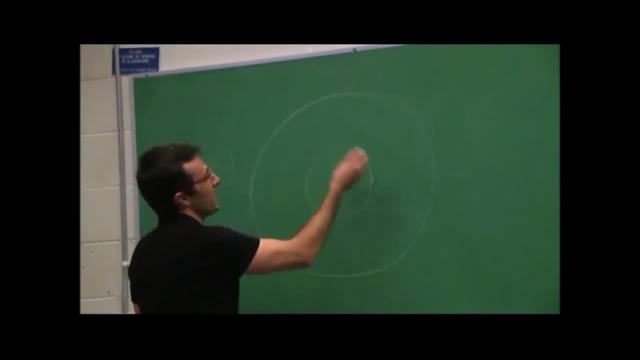 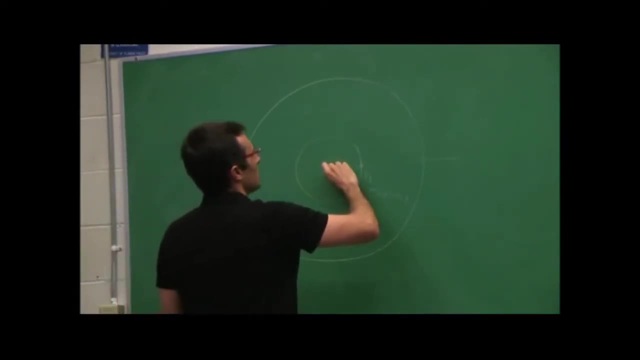 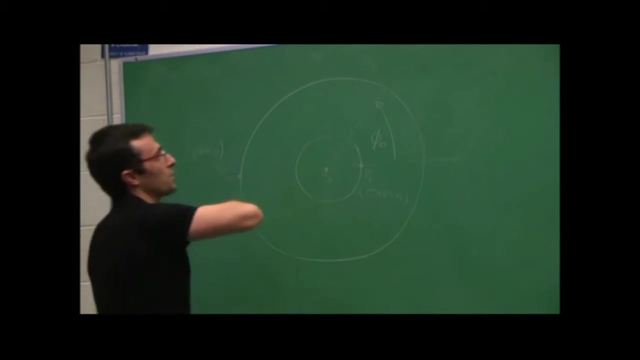 So we were dealing with the phase angles, how these planets have to be positioned with respect to each other, so that you can do this. So in the previous video you have, You know, the discussion about what this phi zero has to be once you have radius of the first planet's orbit, R1 and R2, which also mean that you have their angular velocities. these are all circular orbits. 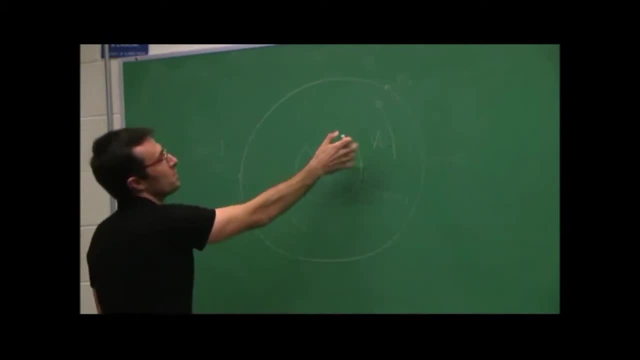 So you know you can compute what this needs to be, so that once you leave planet one and you travel on this half ellipse and you spend time. So you know you can compute what this needs to be, so that once you leave planet one and you travel on this half ellipse and you spend time. 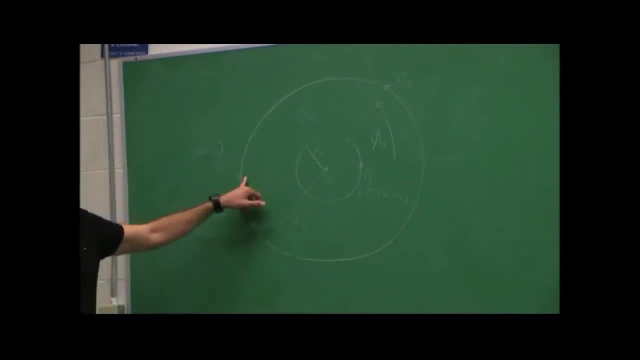 So that P2 is going to be actually at the apogee of the transfer, right. So that's a simple angles exercise that you should have seen in that video, And I believe there's also discussion about how often you actually see the right phase angle to do a Hohmann transfer from one to two and I believe between Earth and Mars is about two plus years. 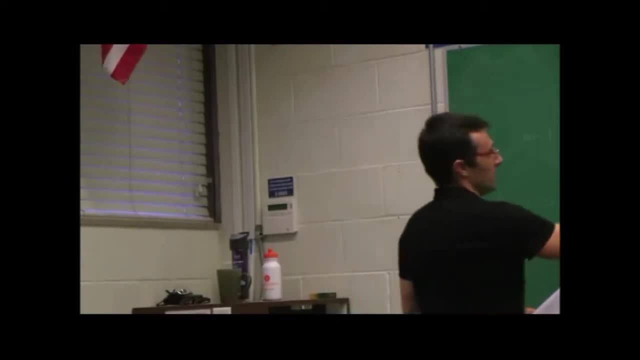 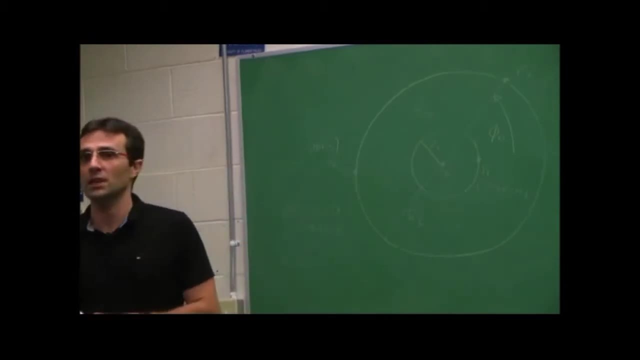 So that's how often you can have the right configuration, like in this case For phi zero, so that they actually your spacecraft is actually going to meet Mars at the other side of the ellipse, right? So if you miss the window, you wait. 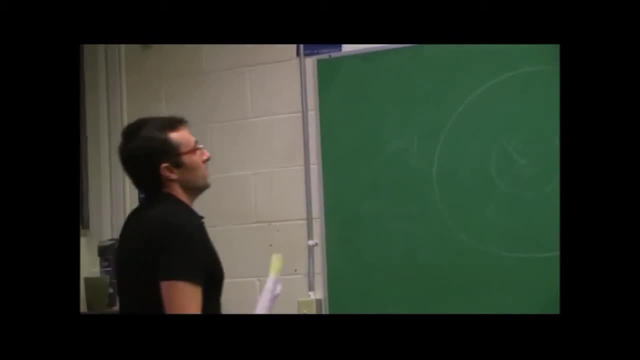 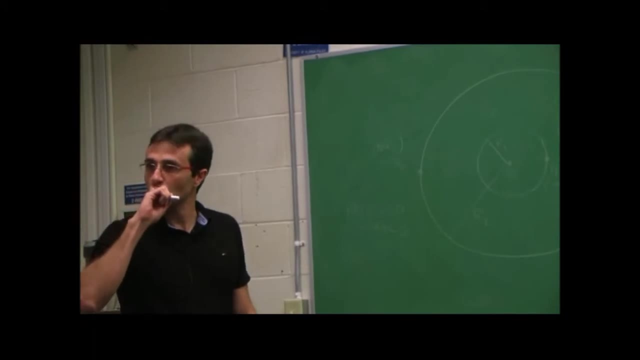 For this kind of maneuver. of course it's not the only one. You know it's an impulsive, the most efficient one. You have to wait more than two years. Yes, Would that like have you crashing into the planet, or like starting to rotate it? 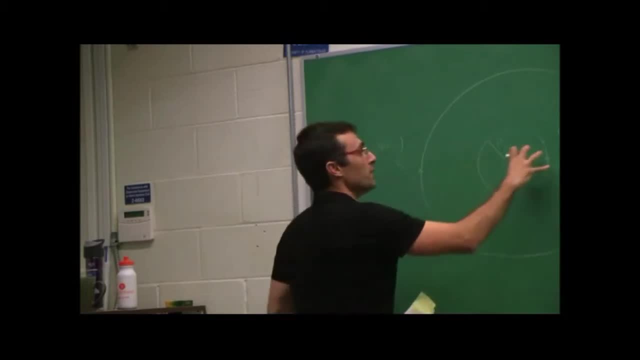 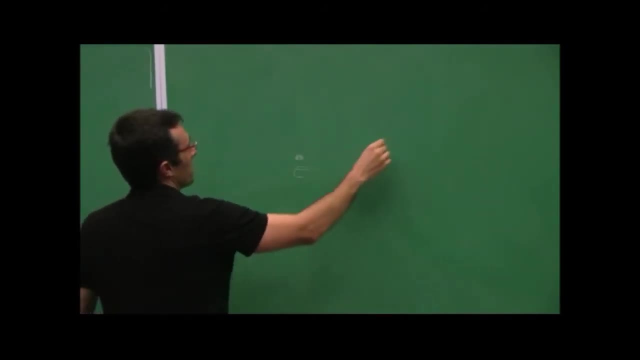 No, no, no. So these kind of again, these are patch conics. So if I zoom in, for example, around P1, what is actually happening Before I leave the sphere of influence is that, and again, P1 is my planet Earth. 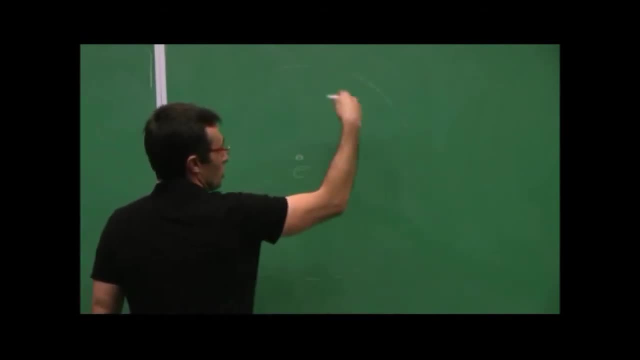 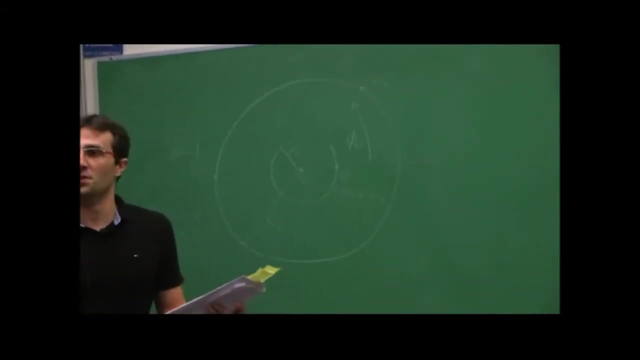 I have this imaginary volume around the planet- We'll compute its radius today- And inside that volume, I can assume that the only attraction that I experience is the Earth. I don't care about the sun, I don't care about the moon. 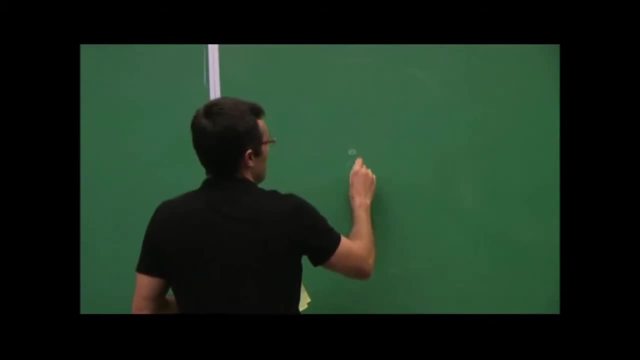 It's an approximation, But that's all I see. So what you're actually doing here is that say that you're- And we'll see these in the next lecture- actually Say that you're on a circular orbit around the Earth and at some point you're still ready. 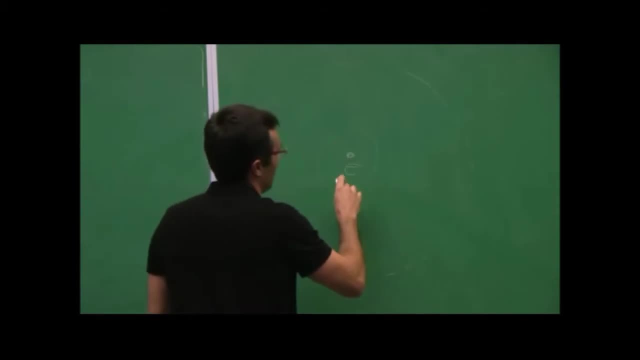 You time this Correctly. you need to get out and go on the transfer ellipse. Well then, you're going to probably burn here, so that you go on a hyperbolic path with the right asymptote that leads you at the edge of the sphere of influence. 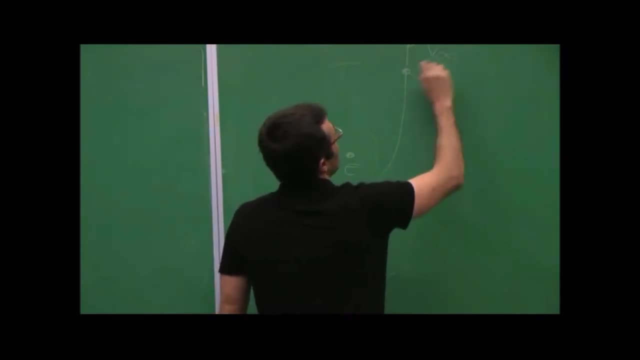 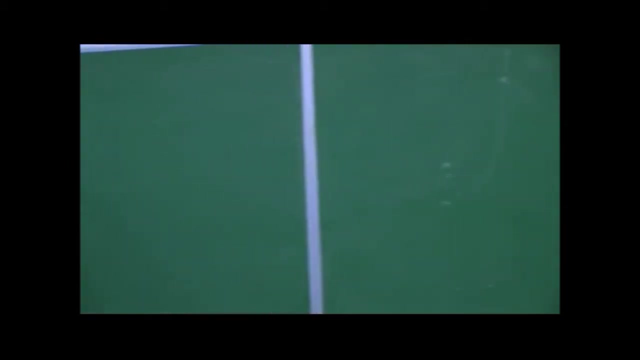 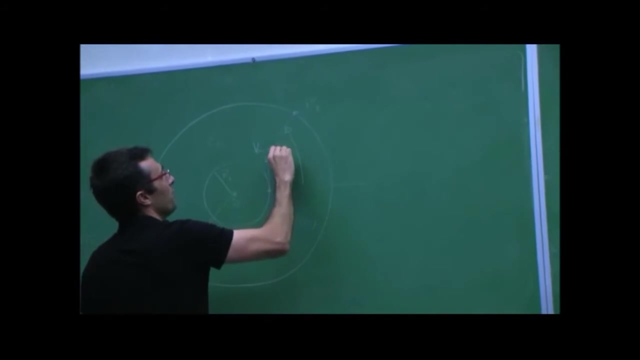 with some residual velocity that is sufficient, so that you sum this up to the velocity of Earth. And now you go outside and from the sun's perspective, here you're going to have V infinity. this is the velocity, V infinity plus V, of the Earth. 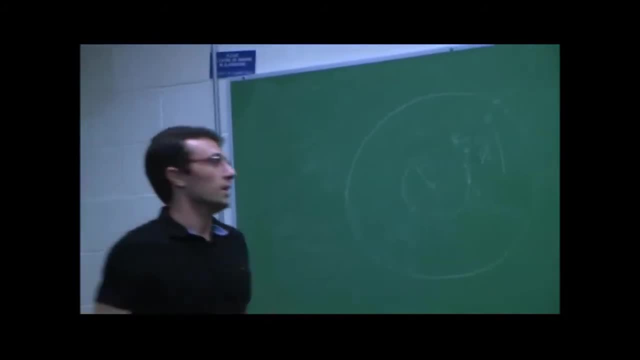 Because, remember, everything we've done so far is relative to the planet. So, if I am inside the sphere of influence of the planet, everything that I'm doing is relative to this planet, and this planet is also traveling with respect to the sun. 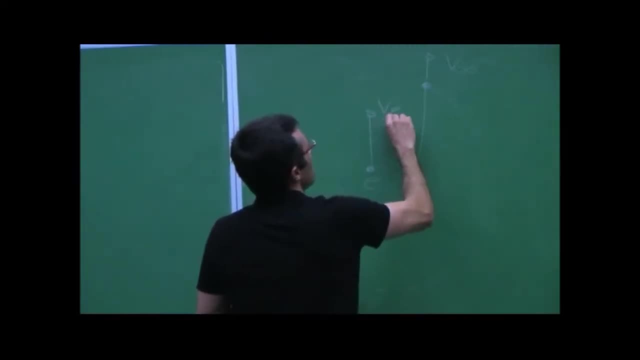 So this planet has its own velocity. So what you're doing here is you are burning here so that you go on the right hyperbolic path, such that the excess velocity adds up to this and you have the right perigee velocity. 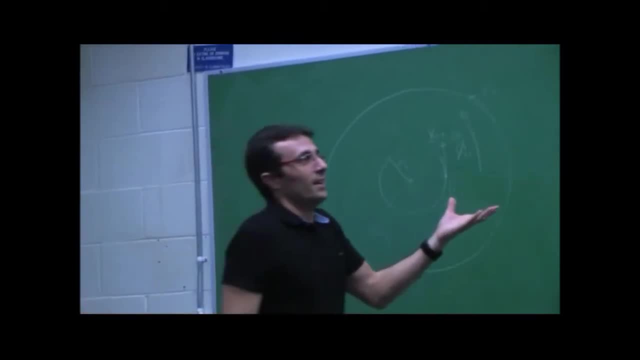 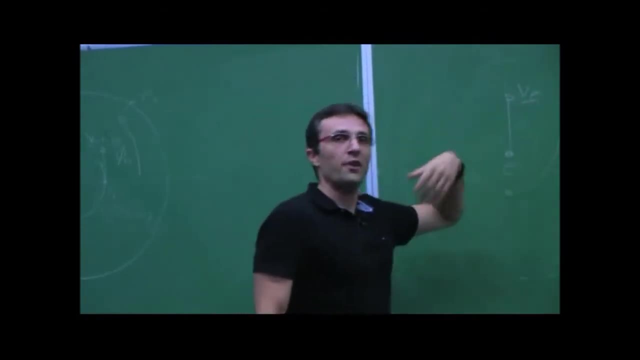 with respect to the sun. That's why it's called patch conics, because it's not actually what happens. I mean, you are always under the influence of the sun as well, but here I'm just saying, hey, when I reach this distance, here I forget about the Earth and all of a sudden all. 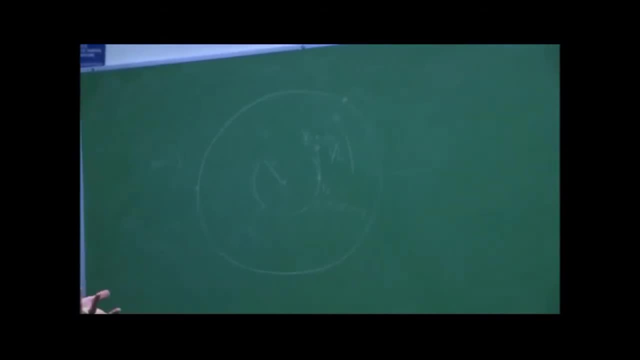 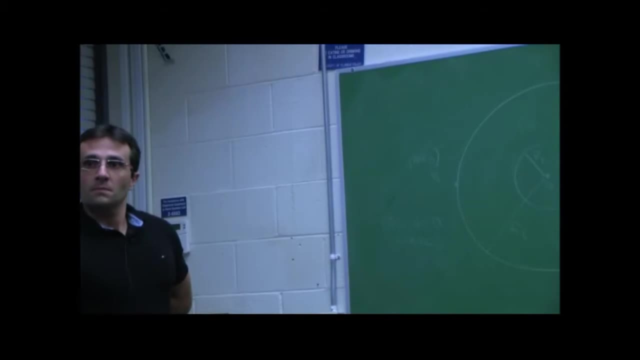 I see is the sun. It's a rough approximation, but it gives me an idea of the delta Vs that are involved. Yes, So in that sphere we just worry about the full force of gravity from the Earth. Yep Right. 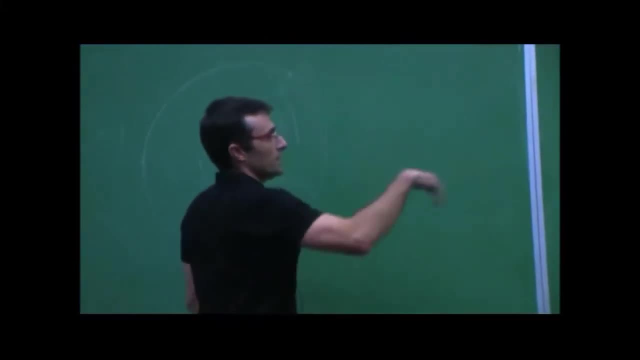 Right. So if you have to look at all the equations that we've seen inside the sphere of influence right here, you only care about using the mu of the Earth, Right. Once you leave this thing, all the equations that you're going to use only have the mu. 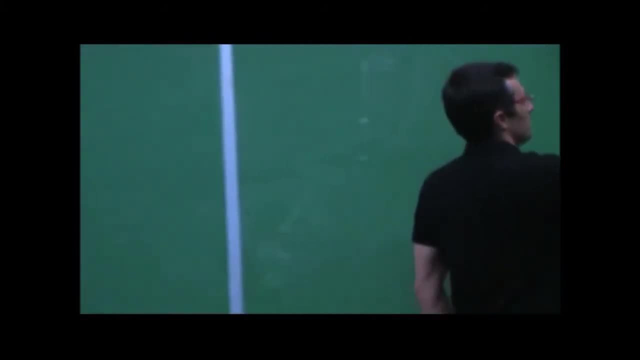 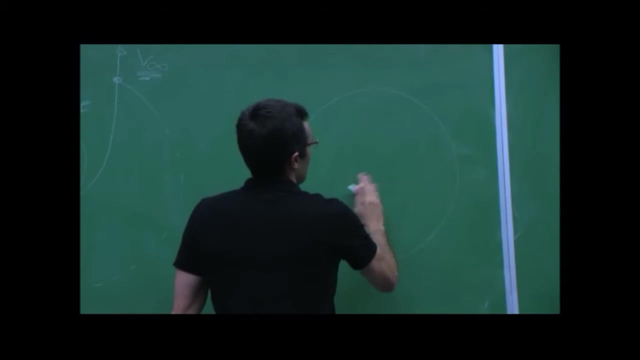 of the sun until on the other end- this is Mars- It's going to have its own sphere of influence, which is a little smaller than Earth's, because it's a function of the mass, as we'll see. And so here you're actually coming in with some velocity. that will be your V infinity. 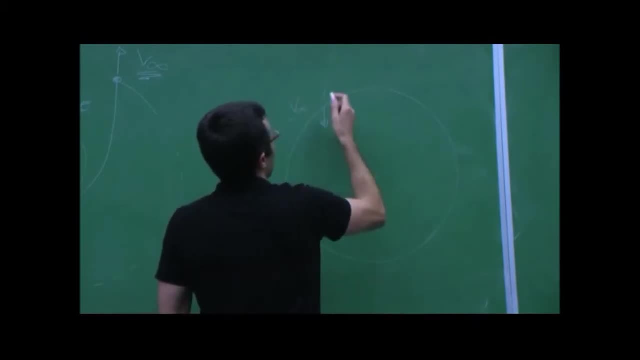 but now you're coming in with that velocity. It's a different one. This is whatever that is, And you're coming in with this hyperbolic path that, if you don't do anything, you're actually going to exit on the other side. 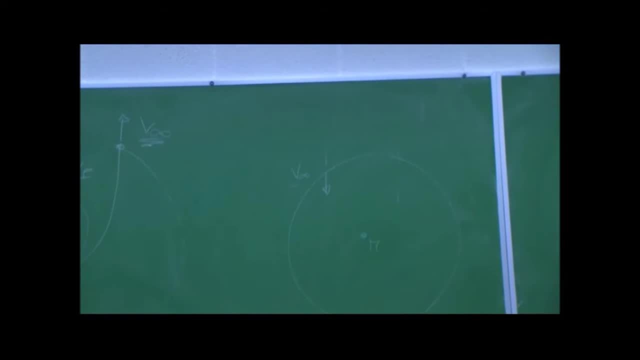 But obviously, if you want to remain there, you will have to slow down and go into some circular elliptical orbit around Mars. So this is the idea of patched conics: I do something around the first planet so that I have enough V infinity to leave its. 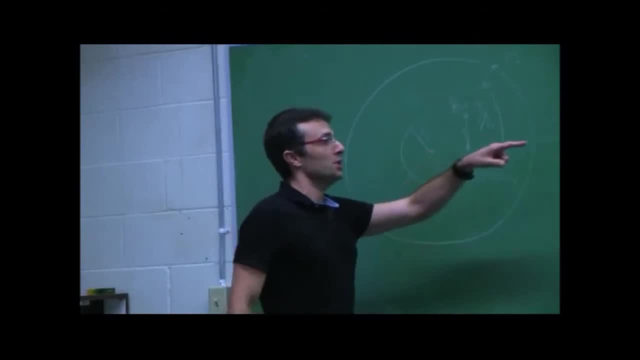 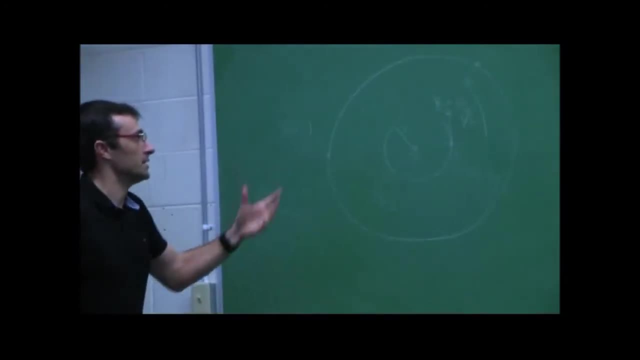 sphere of influence and I will add that velocity to the inertial velocity of the planet with respect to the sun and that gives me the total. We'll see this next time, But that is the idea. That gives me the total velocity. that is enough to go on this. 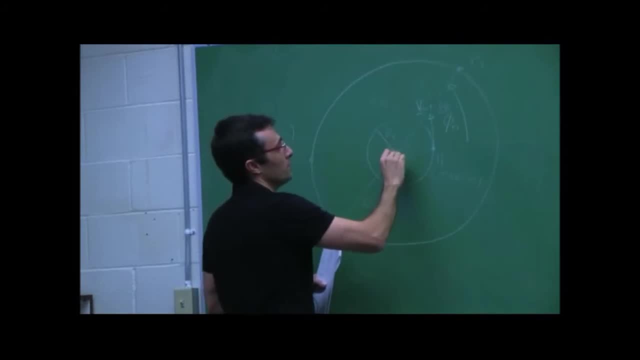 Half ellipse that is only based on mu s, basically on the attraction of the sun, until I get close enough to Mars that I'm actually switching to its sphere of influence. So you don't care about. basically you're still doing single attracting body kind of. 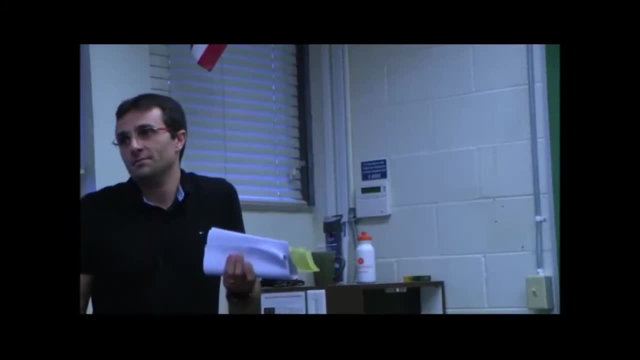 astrodynamics, You don't do two at the same time. That is the approximation that it's using. Make sense, Is this approximation good enough for actual orbits, or is that just? It gives you a ballpark number for the For the delta v's that you have to use. That's basically the idea. Yeah, Then, if you have to do it precisely, you definitely have to have some software that takes into account, like the spice toolkit that Patrick discussed, that actually takes into account the gravitational attraction of all planets at the same time. But you know, if you look at the What happens in lower orbit, the attraction of moon and sun, as we have seen, they're really negligible with respect to J2 and drag, for example. So you know, So it really depends on distances. 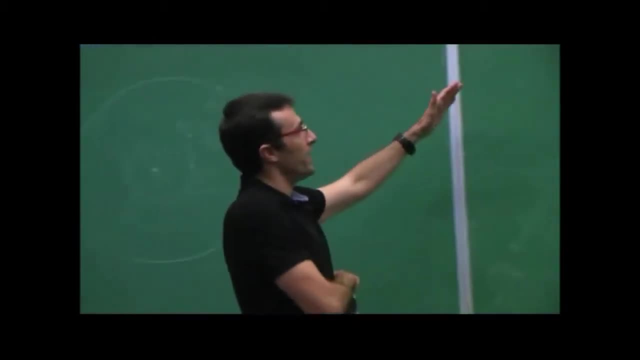 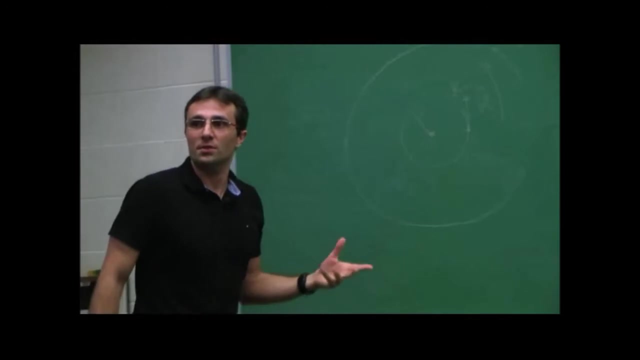 Of course, as you get closer and closer to this imaginary edge of the sphere of influence, the approximation that you only see the Earth as the attracting body, it's losing its power Because the Earth becomes smaller and smaller. you're going away and you probably start. 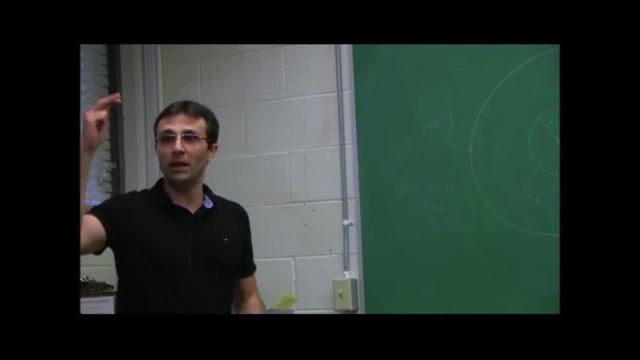 experiencing the attraction of other objects: The sun. if you look at the masses of the planets in our solar system, the sun is, I want to say, three orders of magnitude or more More massive than Jupiter, which is probably three orders of magnitude more massive than. the Earth. So the sun is dominating everything. So it's, of course, an approximation that loses its power when you leave all these smaller objects around the planets, But it is used. It is used for ballpark numbers in terms of delta-v's. 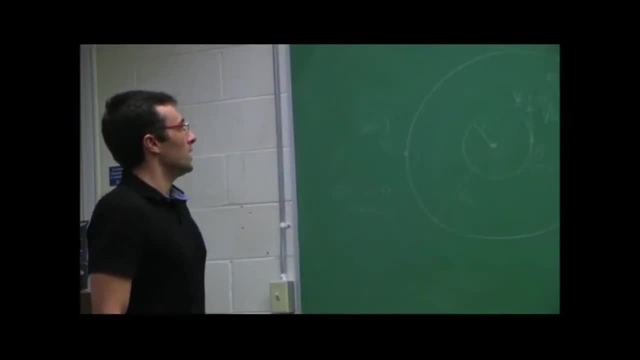 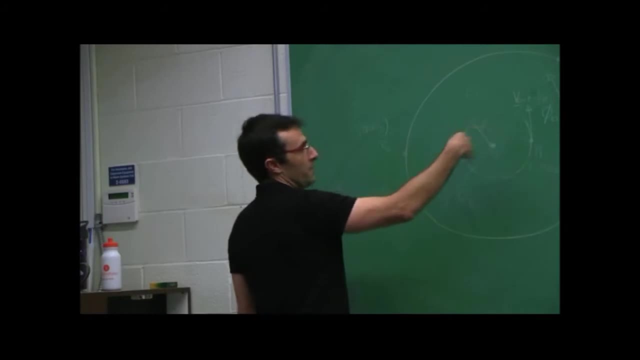 So what I needed to finish, though, is: well, we know that these, the correct phi zero to transfer on these half ellipses, is every two plus years. Now imagine that you have reached Mars Somehow. you slow down, you remain, you land on Mars, you do whatever you have to do, and 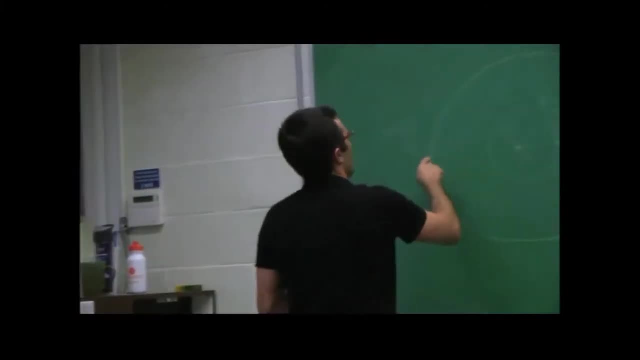 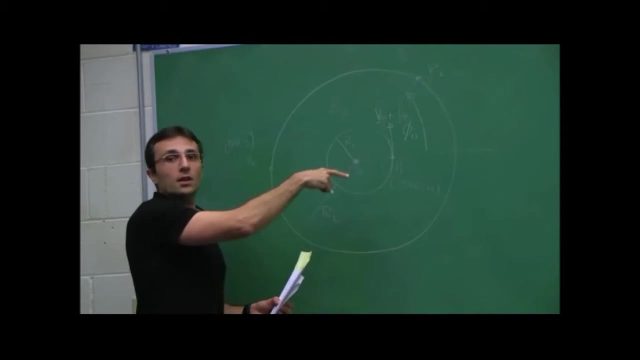 then you want to come back. First of all, if I just wanted to reach Mars and come back right away, you can't just remain on these ellipses and hope that planet one is going to be right there, of course, Because what happens is that planet one, and I didn't bring my computer because I didn't 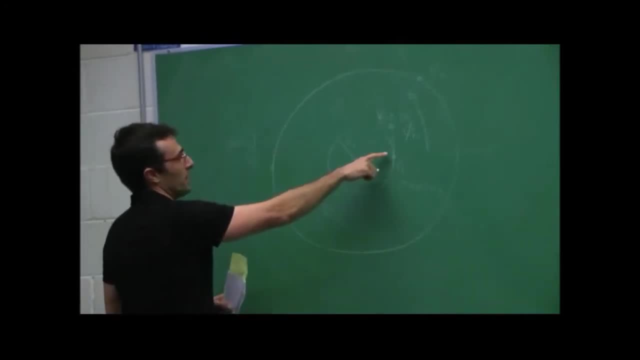 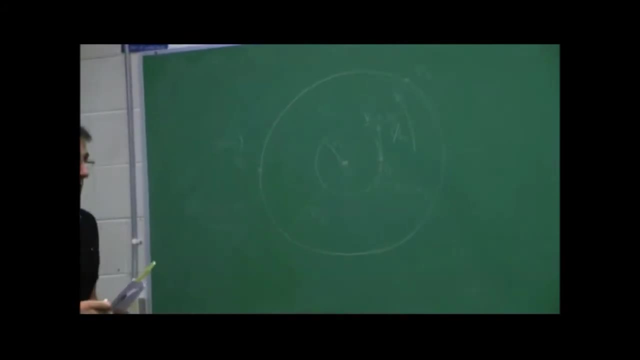 want to carry a backpack, basically. But think about this: The planet one is on a smaller circle, so that means it's moving faster around the sun. By the time the spacecraft has reached Mars, in this position, planet one would be somewhere. 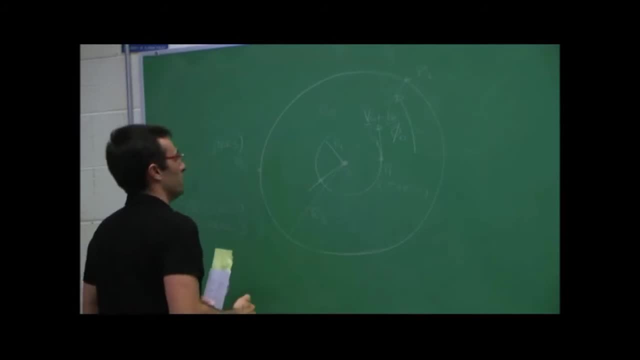 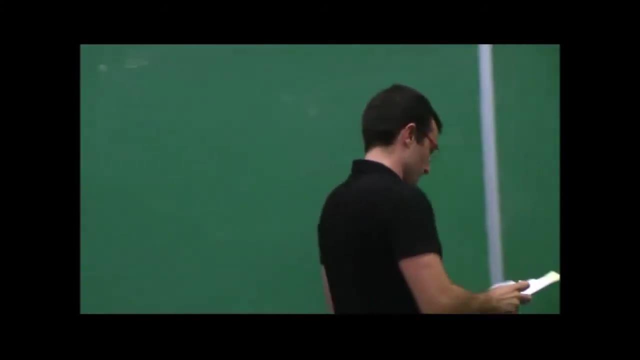 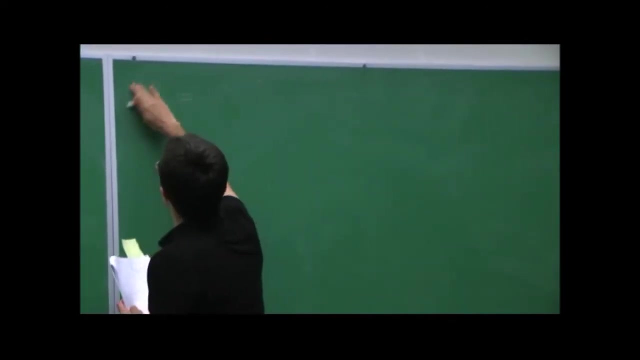 here It would be ahead of planet two in terms of phase angle In particular. if you look at the equation for the phase angle- I think this is also the end of that video- You can easily compute that the final phase angle. so at the end of that T12 transfer. 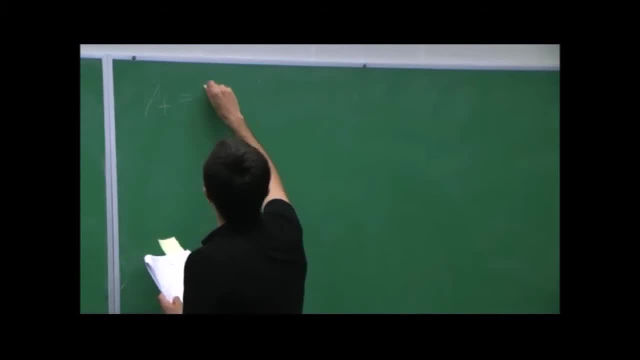 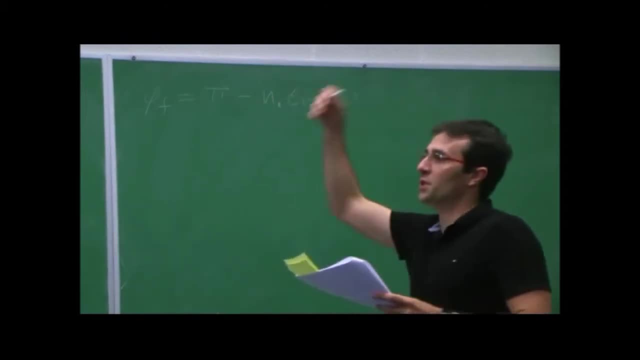 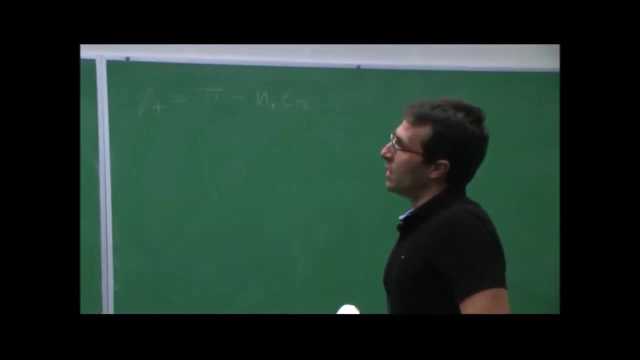 ellipse, the actual phase angle between the two planets is pi minus n1- T12.. Where n1 is the angular velocity of the Earth around the sun. in this case, If that's P1, if P1 is the Earth, So you can easily prove to yourself that this is actually negative. 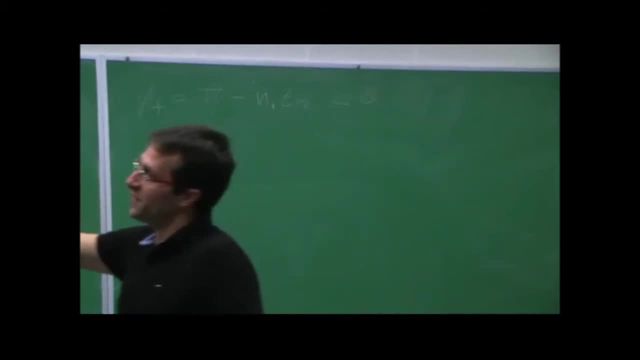 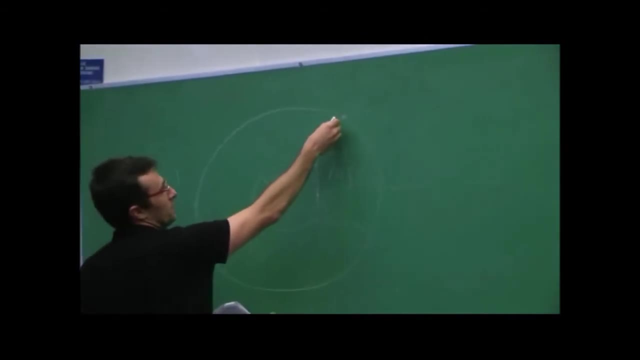 negative, which means, by the way I have defined the phase angle, which is the angle of. so this is my line of reference to measure angles. the phase angle that we define is the angle of P2 minus the angle of P1. so if that's negative, it means that planet 1. 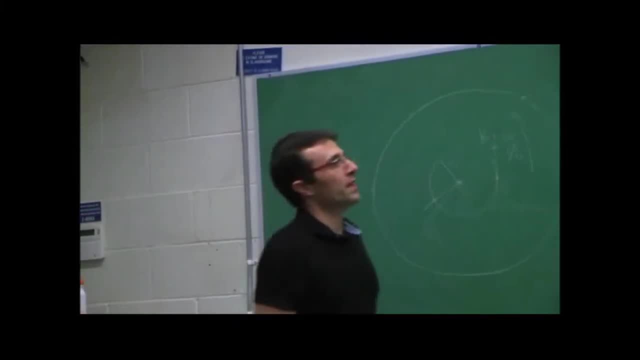 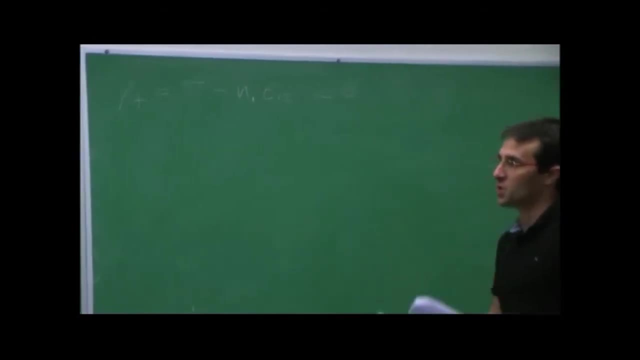 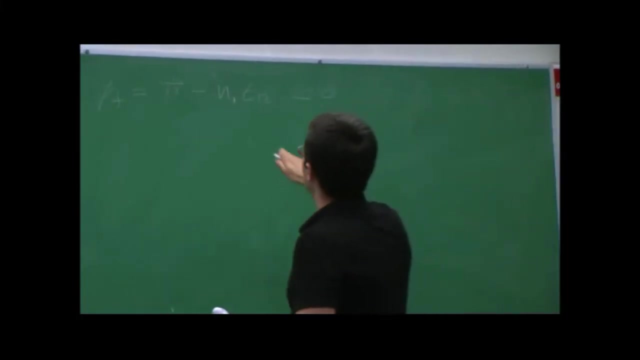 is ahead of planet 2. how do you prove that? well, again, think about what you have. T12 is half orbit of P2 on the ellipse that has the same major axis, which is bigger than the same major axis of planet 1's orbit, which is R1. so you can easily see. 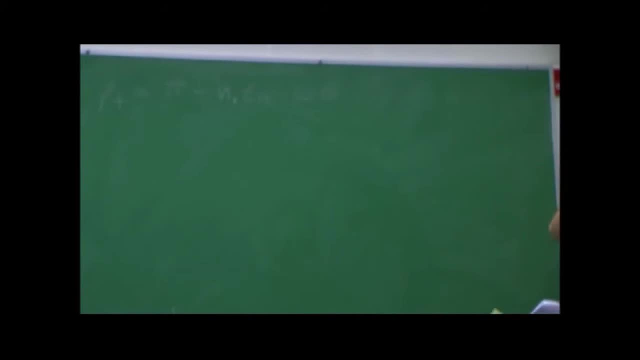 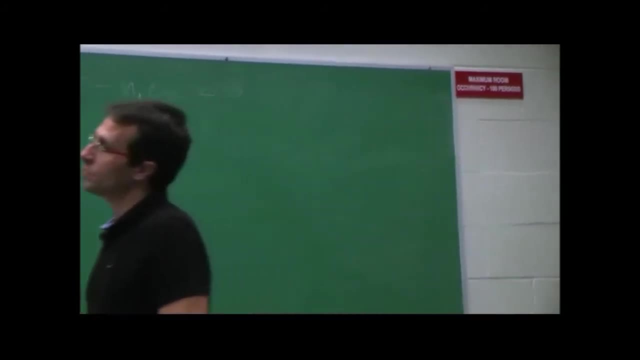 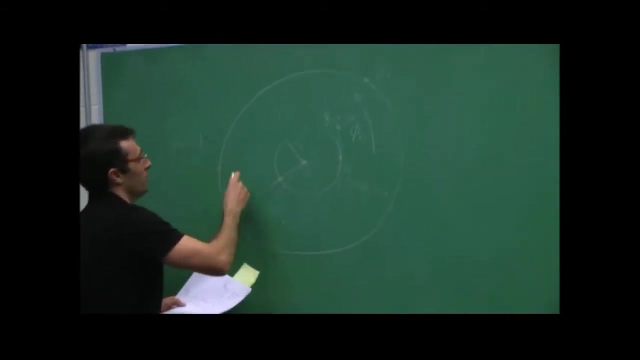 that this is bigger than pi. anyways, it is negative. so what do I want in terms of the next phase angle? well, I want to know when I'm good to actually leave Mars, basically run the same exact ellipse, just the other half, if you want. of course, it will be somewhere. 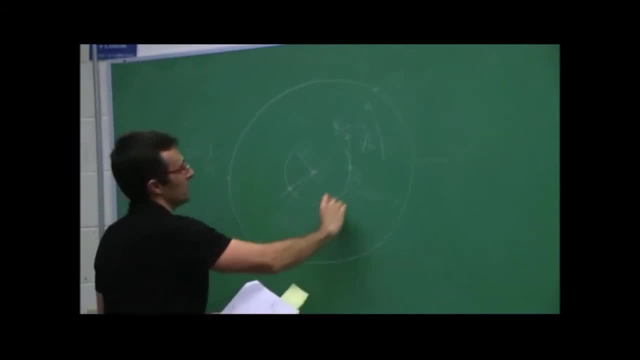 down here. it's not going to happen right away, but the sketch is still valid. you're going to run these other half ellipse and have planet 1 at the right location and the time of flight is the same right. I'm using the same kind of ellipse. 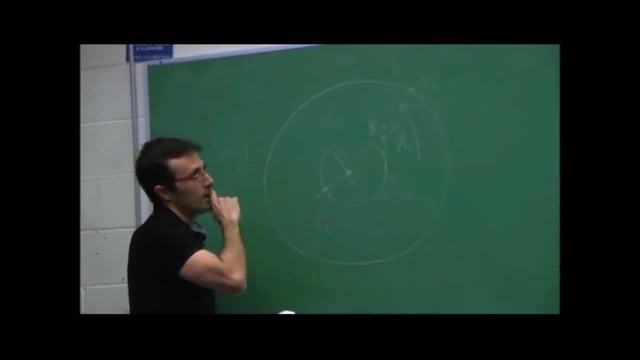 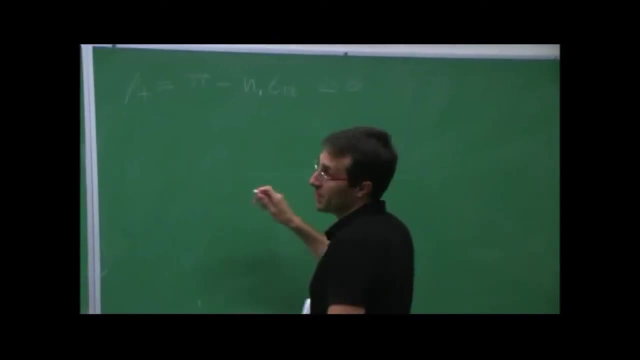 right, this is to get there and this is to come back. so what has planet 1 done? planet 1, if I redraw my line to measure angles- and this is the can't draw circles, of course, this is my circular orbit of planet 1. I left from here. 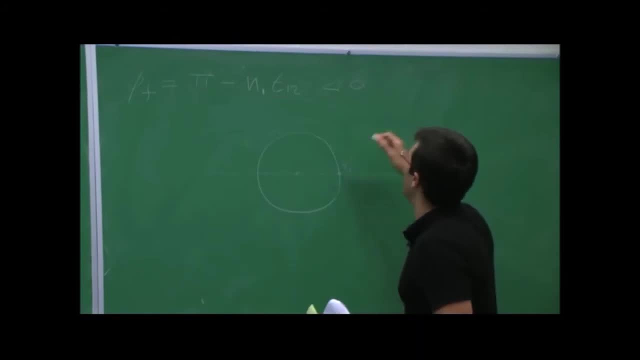 so let's say this is p1 prime. you know, at the moment of doing the first, delta v going on the ellipse to transfer. so it will travel on its path and then it will end up somewhere here where this angle is my new phi final right, because this is where I want. 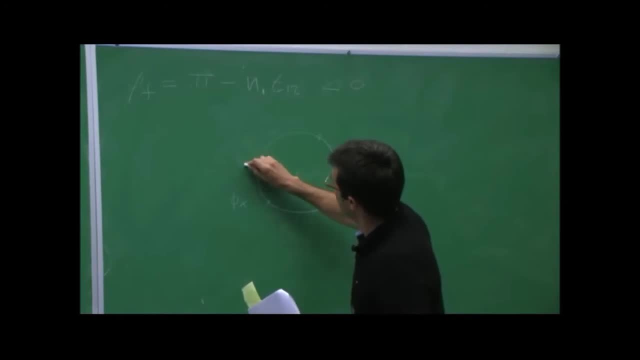 planet 2 to be at the end of the transfer. so this is planet 2, second at the end of the transfer and this is planet 1, second at the end of the transfer, does it make sense? if you want, I can draw also the bigger circle here. 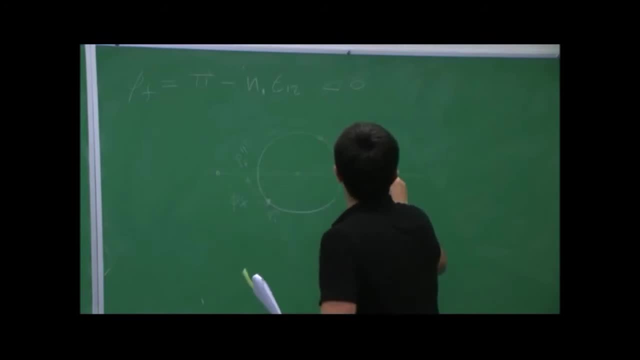 because planet 2 is actually not here. yeah, it's, it's somewhere else here. so, yeah, on the bigger circle, right, bless you. so, and this was planet 2 at the beginning of the transfer was here. it travels lower than planet 1 on its orbit and it ends up here. 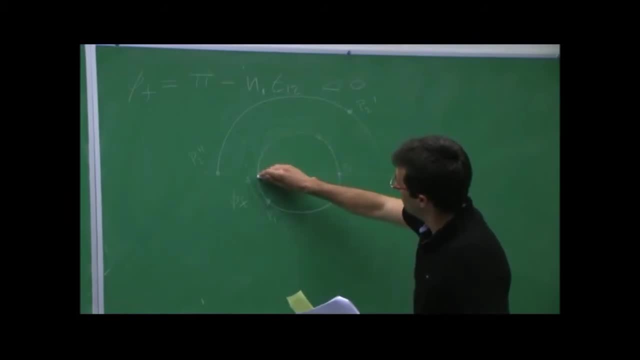 and in the meantime, planet 1 goes from here to some position down here that is ahead of 2, given by this angle, right? so what I want is is basically to find my planets in a new initial phase angle so that planet 1 can travel another. 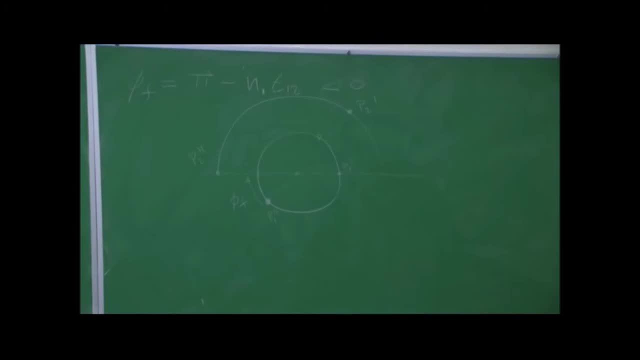 pi plus phi. final right: it has to cover the same distance on that circle. so this is the same distance on that circle. in other words, you need to wait for a new. call it initial phase angle. I'm calling it phi zero prime and that needs to be minus. 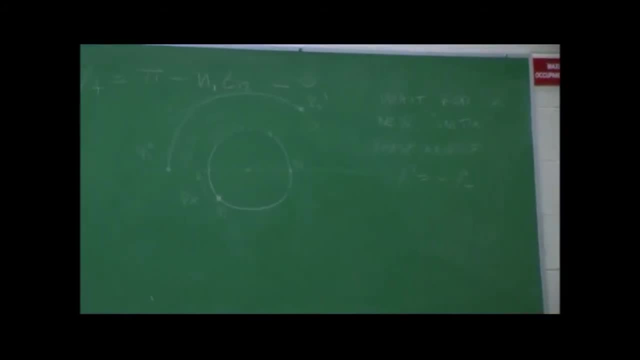 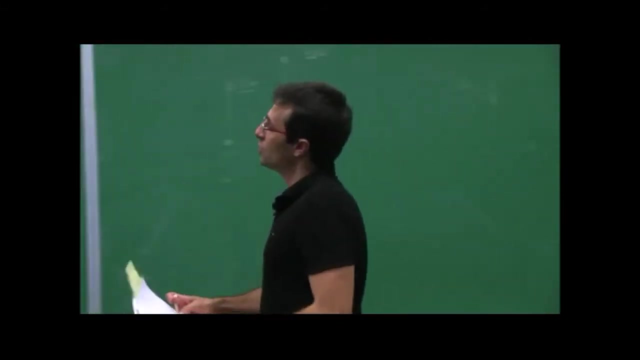 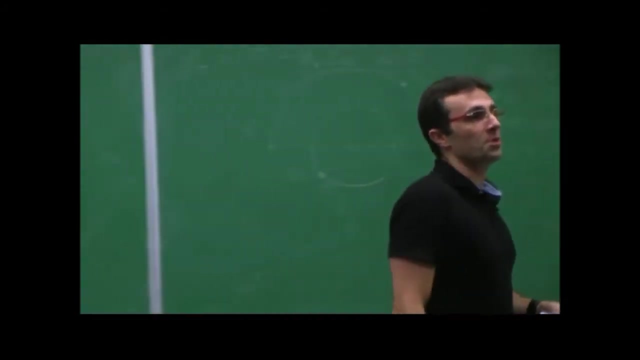 phi final. does it make sense? I need what I had. there was actually planet 2 being ahead, right? so I need to wait enough time so that these two objects find themselves in a configuration where planet 2 is ahead again. otherwise I'm going to have to wait for the next one. 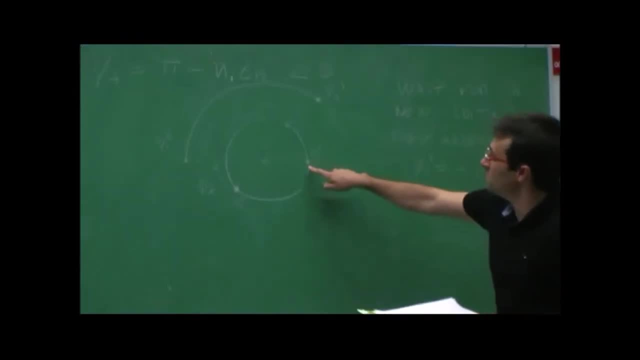 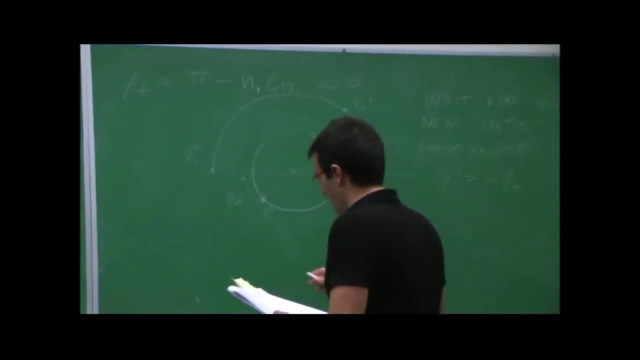 so I'm going to have to wait for the next one. the moment I leave it, I cannot expect planet 1 to be where it needs to be. can we see that? alright, if that's what I want, then I go back to my phase angle equation. that was. 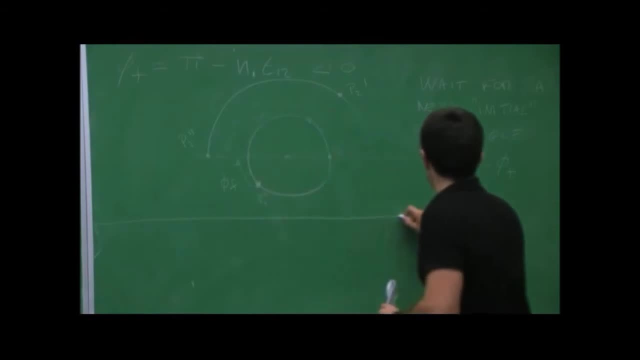 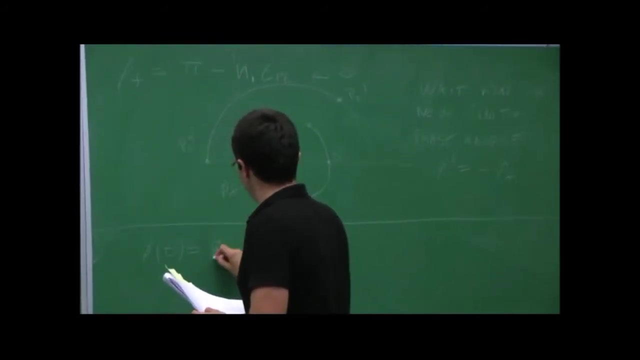 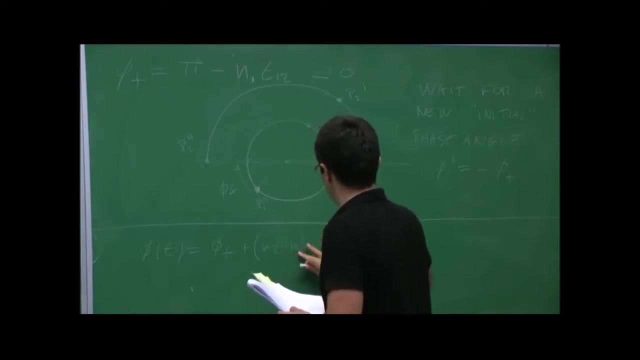 yeah, the general equation was phi as a function of time. now my new initial condition now is phi final, because I'm starting to count from there: plus n2, minus n1 t. this is something you should have seen in the video, but I know that I want to find the time. 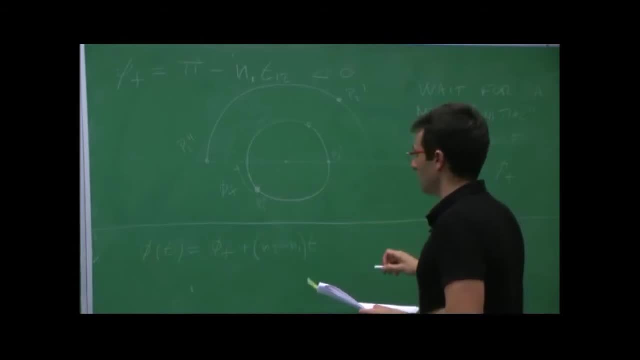 the right time so that that phi becomes minus phi final. so I'm going to substitute this in my desired angle, so I get plus n2 minus n1 plus n2 minus n1 plus t. so now you have an equation where I know what this is. 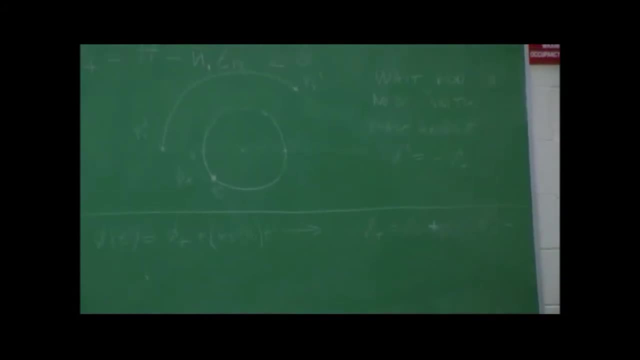 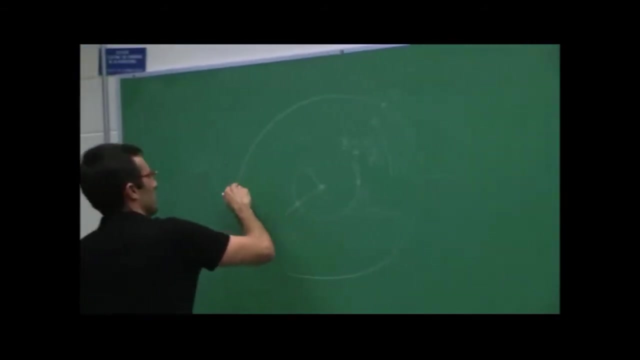 by the way, I can always plug it in. I can do it later. I have an equation where I can solve for my wait time. so, again, what I want to find here is after I leave. I have left planet 1, I've gone on this ellipse. this is the time. 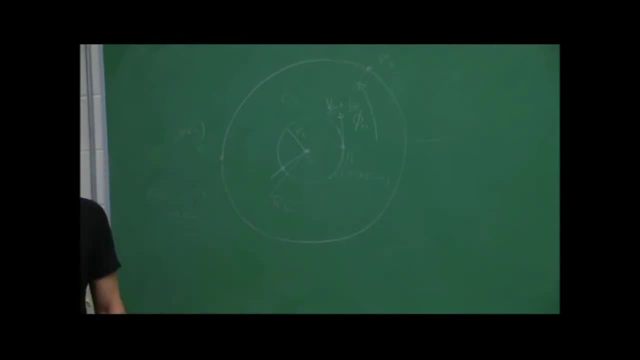 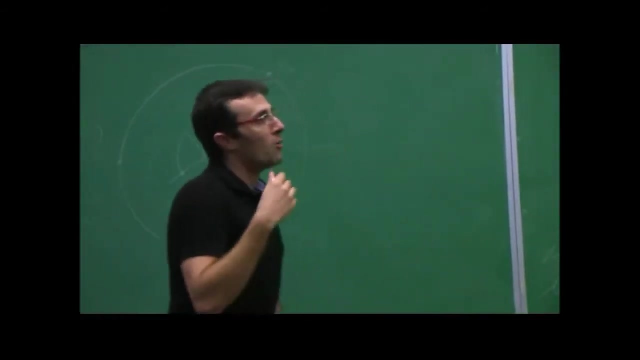 where I reach planet 2, I reset the clock right there. so that's my new 0, right. i start counting time from there. that's what i'm doing. so from that point on, i want to know how much i have to wait so that the planets are in a configuration where i can. 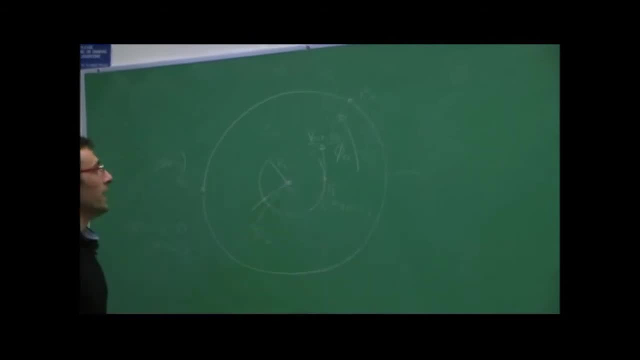 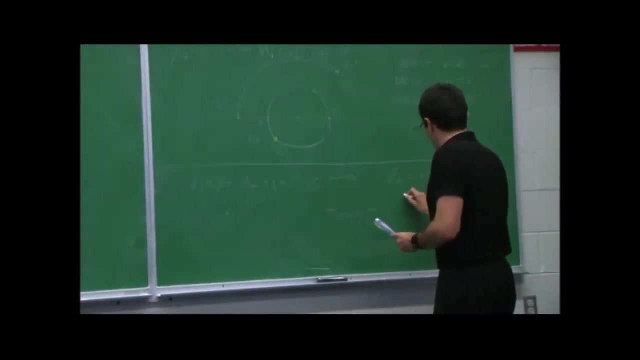 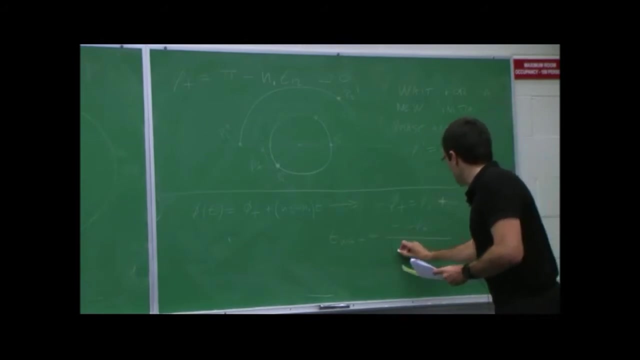 run a similar half ellipse- it's identical basically- and find planet one at the other end. okay, so t weight here. if you, uh, if you plug in, everything that we have is going to be, of course, minus two phi final over some minus here and two minus and one. 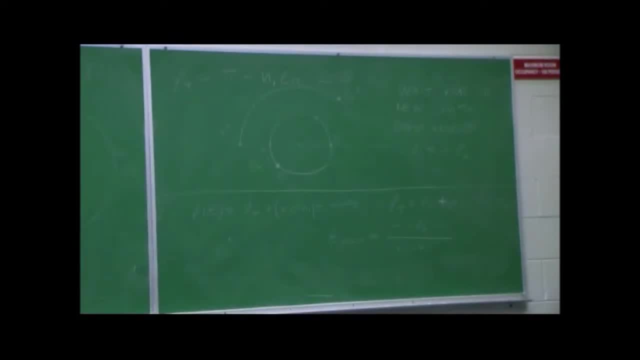 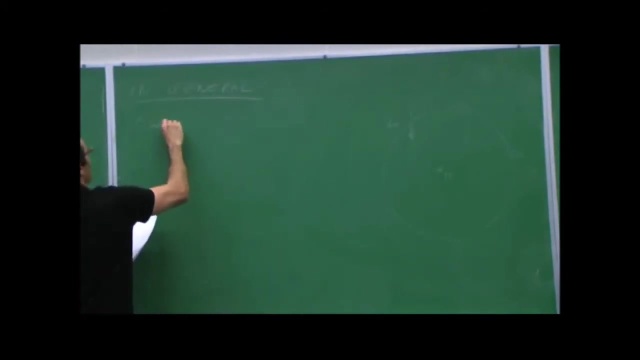 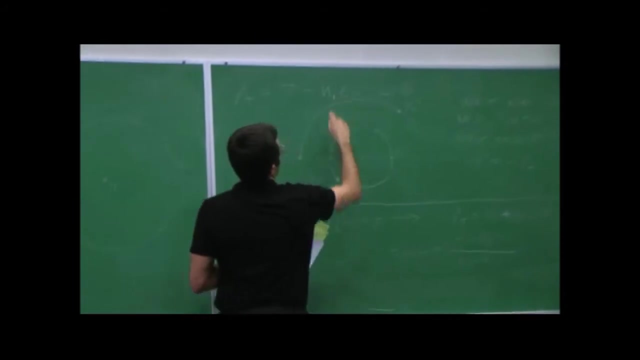 and uh, if you want to generalize, i don't think i need to cancel that in general, so that is the shortest way. weight: but in general you can say that your weight time to come back home basically is minus two, whatever your phi final is, which depends on angular velocity of first planet and time. 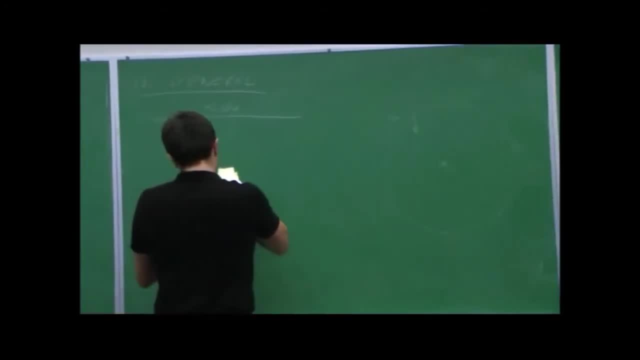 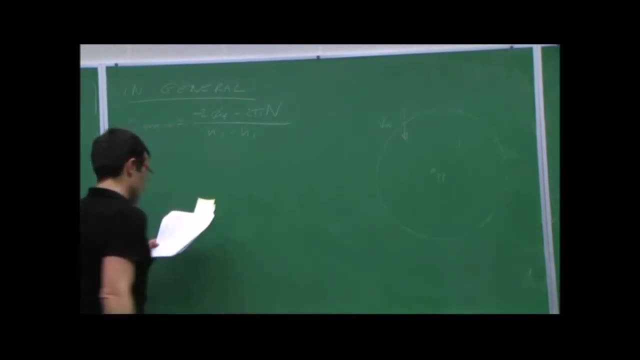 of flight to transfer um minus two pi n, where n is an integer divided by n. two minus and one. and this is again we're doing the case where n1 is greater than n2, without loss of general idea. you can do the opposite. so this is how much you have to wait. you can wait just this or longer, every two pi. 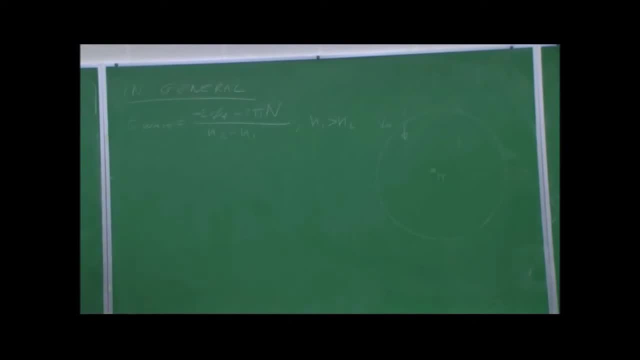 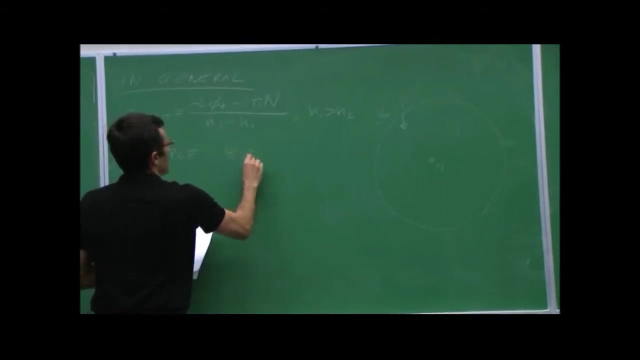 times n? um you're gonna have the planets in the right configuration so that you can return. uh, i think there is an exercise, for example, in your blue, i believe is 8.2, where this is computed um, so that one down there, actually the shortest wait time, is computed between mars and earth again. so they are telling you how. 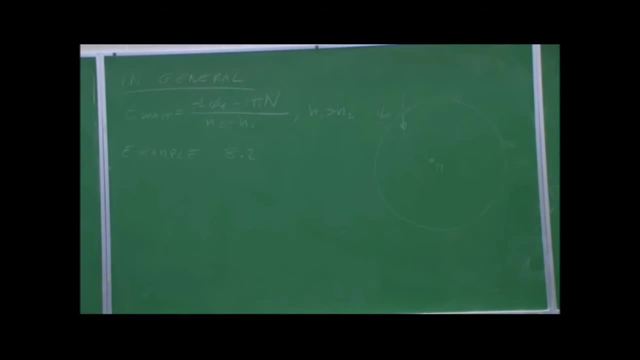 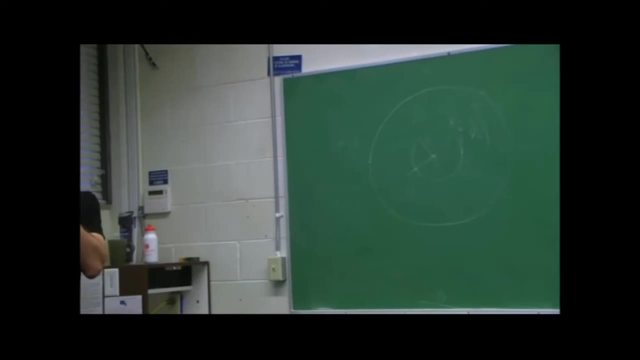 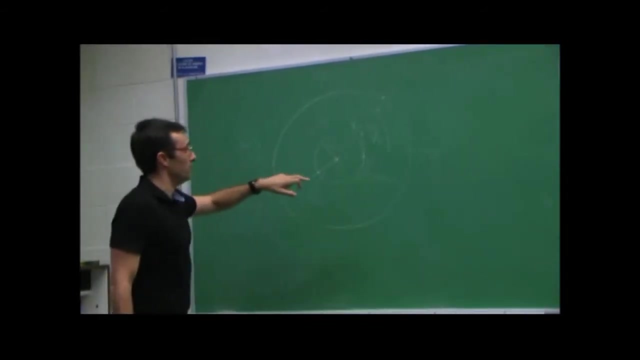 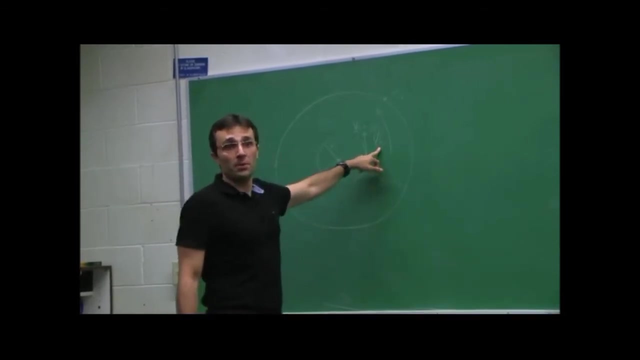 much you have to wait so that you can leave mars and come back, and uh, if i'm not mistaken, i think it's more than a year, 400 something days. so she put all this together, you, you, basically with a home and transfer from earth to march. you wait for the right fee zero to occur, and that happens only more than two years. 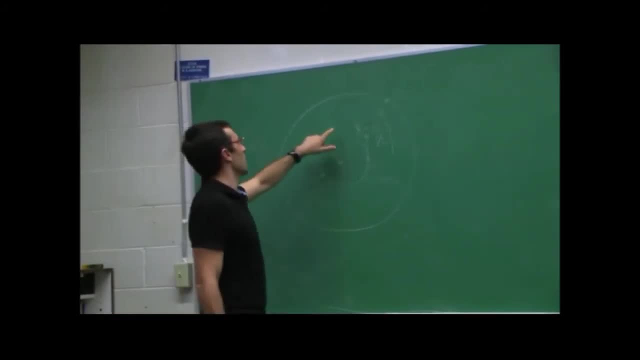 so you, you need to know when you can do it. then you travel on these ellipse, which i think is done, uh, in a previous problem- uh, from monday- i'm not sure what is the travel time that's. it's pretty long, it's more than a year as well, if i'm not mistaken, and then you can't just come back of. 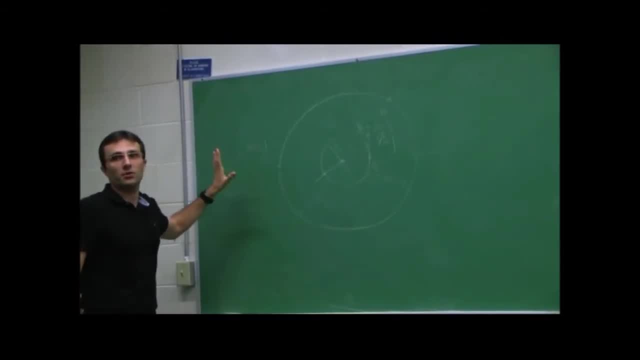 course, why would you want to come back if you're sending a mission to do something there and you have to come back for some reason? maybe there are humans. of course you're not going to come back right away, but the- uh minimum wait time is is more than a year, and then you have the travel back. so 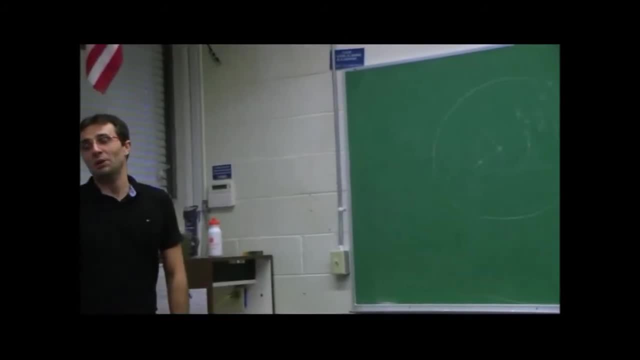 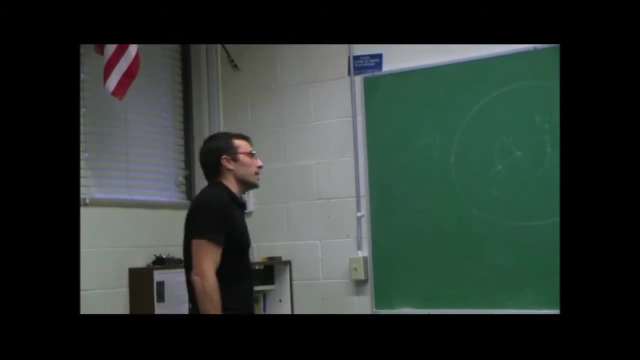 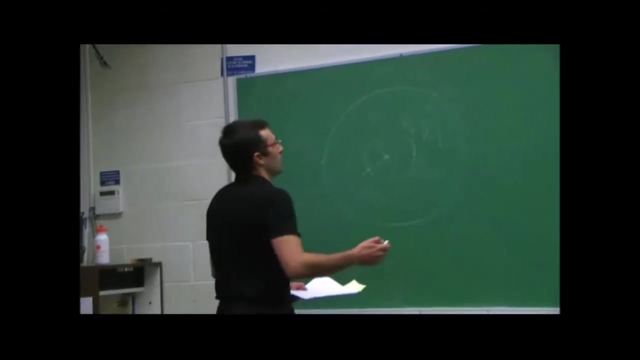 you can imagine. you know you're talking about multiple years in space, which is so far, is a problem for humans. at least it's a problem. but this, of course, this is a homon. two impulse burn. if you have more powerful engines, you can do different things you could. no one is telling. 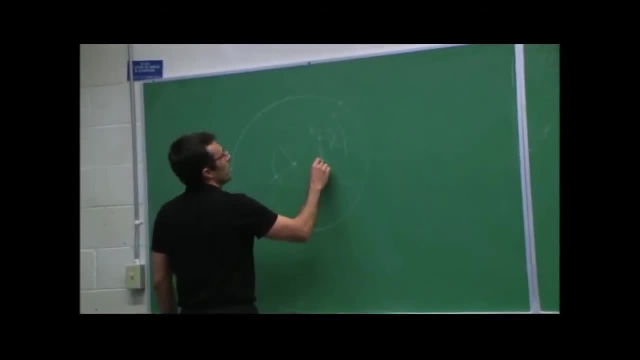 us that you cannot do something like this, where you leave planet one and just go almost in a straight line to planet two and you intersect it here, where the time of flight can be a lot shorter. but that is a function of powerful engines. do we have enough powerful engines? because the delta v's that you're. 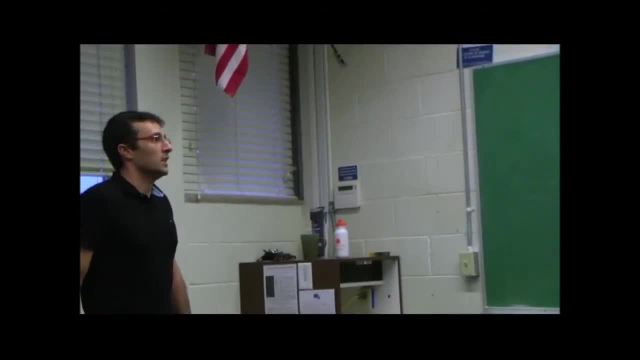 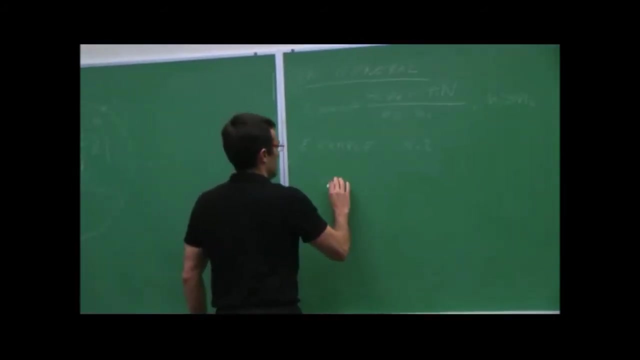 talking about here. take um definitely more than half of your weight just to get there, so you may not even have the right technology to come back um, so yeah, it's expensive maneuvers, that's for sure. was there a question? no, oh, n2 and n1, oh, and, and one is: uh, it's there, it's, it's basically omega. one is the angular. 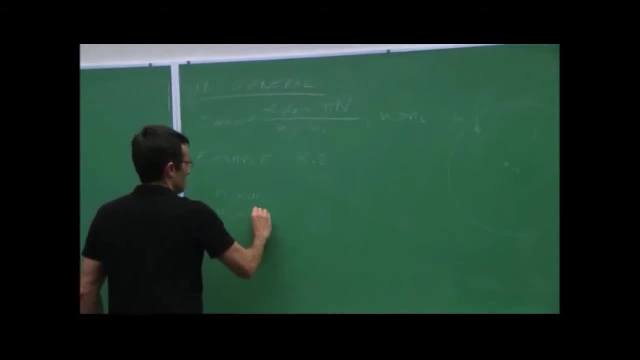 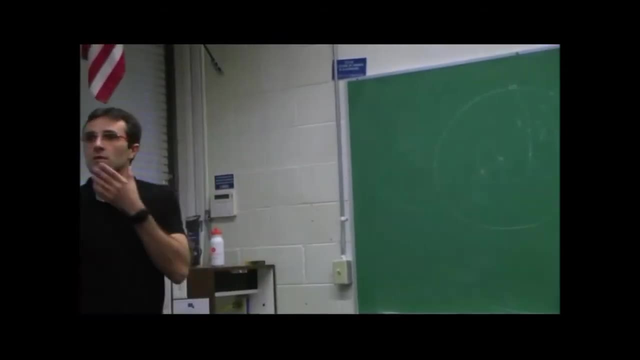 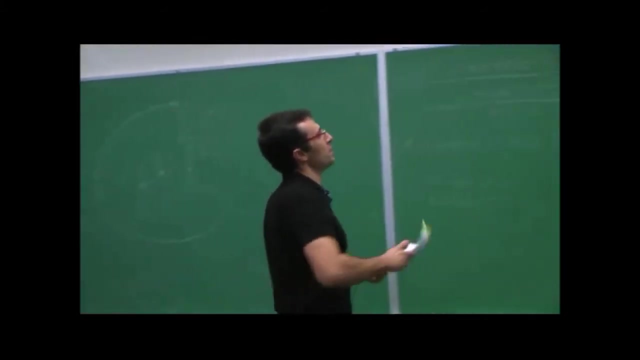 velocity of planet one around the sun, and n2 is omega two is, yeah, proportional to the orbital period of the planets around the sun. yeah, what's the capital? capital, oh, this is an integer. so this is, uh, zero, one, two, three, etc. yeah, because this is all periodic, right, everything, everything repeats itself. um, as a function. 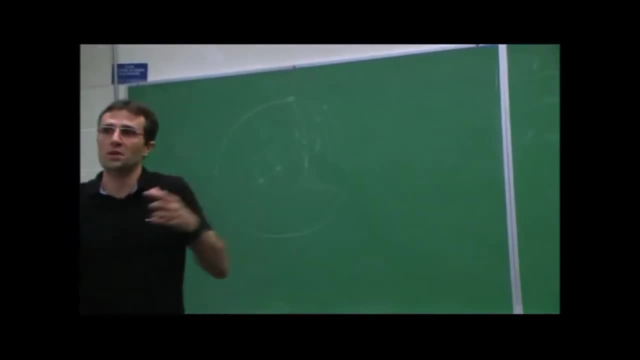 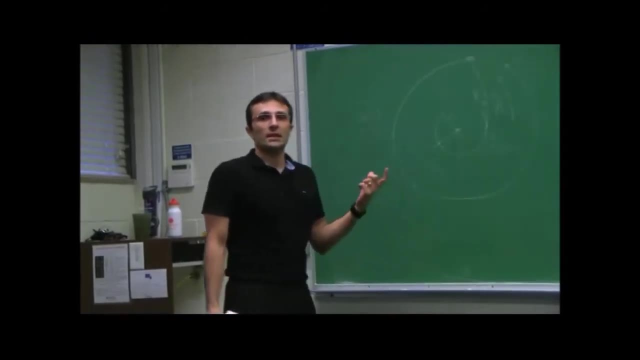 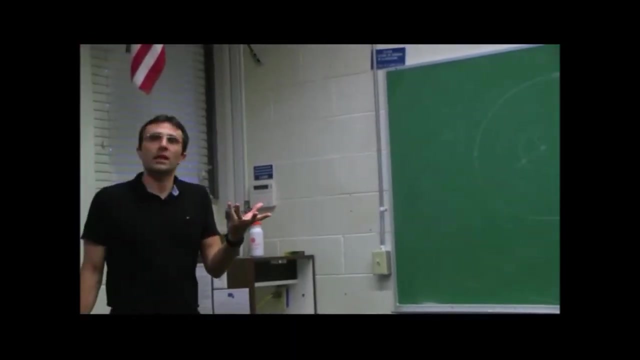 of the difference between these two. they're just secure orbits. one is bigger, one is smaller. so everything that is happening repeats itself, uh, all the time. but it's just a matter of waiting, because these are, you know, our orbit around the sun is what? 365 days or so. marts is a little longer, but 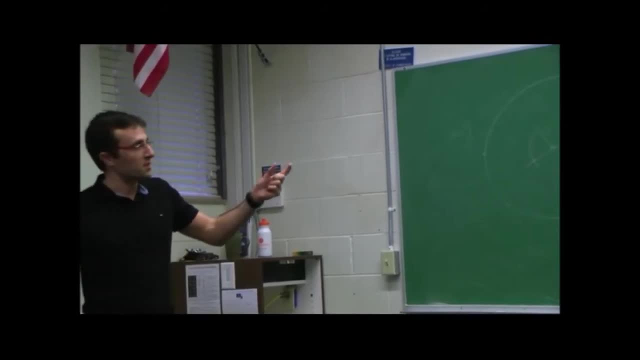 not that much longer. so, um, the difference is pretty obvious. damn it, it's making very big difference here. imagine if it does get smallerし might be all the time, kind of example, to have one night that only makes the z Sol people. so, all right, all right, alright. so if you roughly see like i'm on the moon, but this is what your. 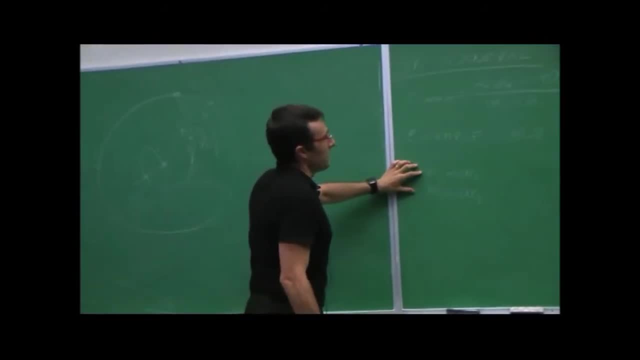 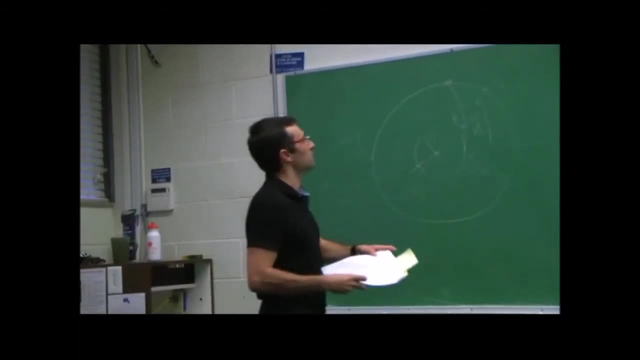 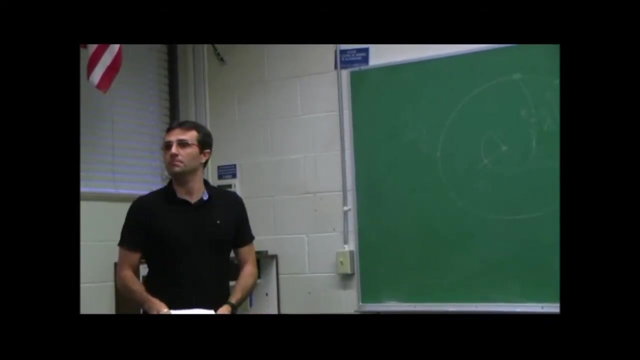 between these two angular velocities is not that big. so that's why you have all these wait times, because before you find the phase angle that you know aligns with the last condition- the same exact condition- you're going to wait, uh, for a long time. make sense. 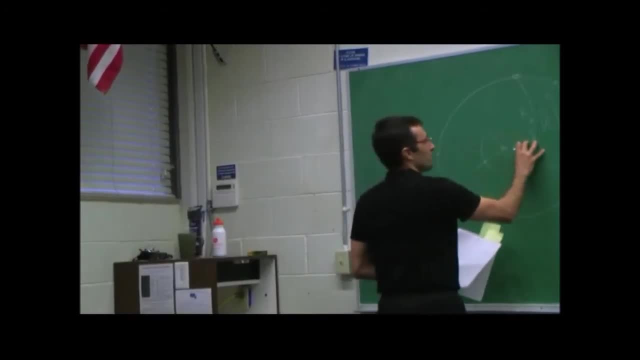 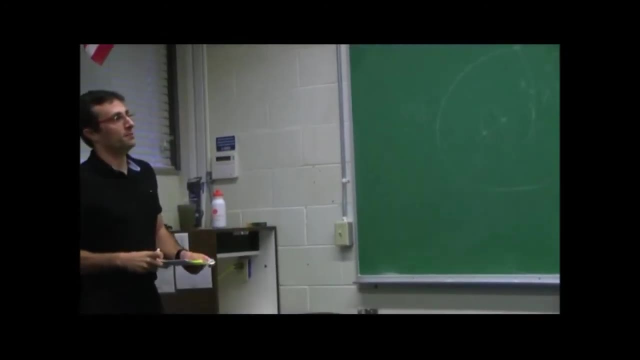 so we'll go more into the details of these. you know what happens here, so that i can create the right velocity and then go on the transfer one, and then what happens at the target planet. but this is, uh, you know, the interplanetary trajectory 101 where you need to time these maneuvers. 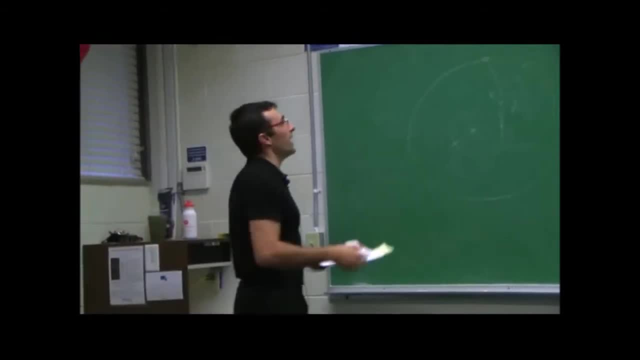 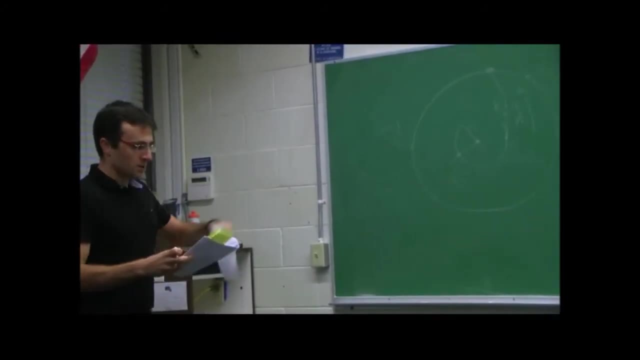 correctly, and you need to know what are the times involved, and this is for the home and transfer, which is, you know, something that we have seen before, so it makes sense to do it that way. now, what is this fuel influence, though? i think it's time to define it. it is: 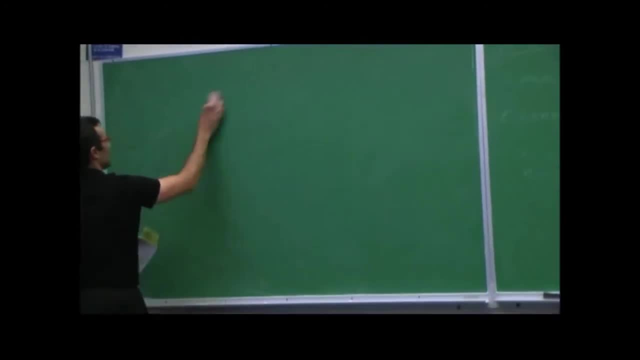 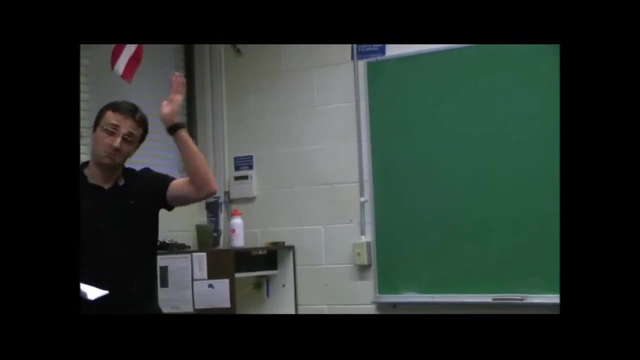 some imaginary volume that we define around the planet, where we say, okay, inside this volume, i really care about only the attraction of the planet, and after that then it's the sun, but there is a way to compute it. so let's say that we're looking at. 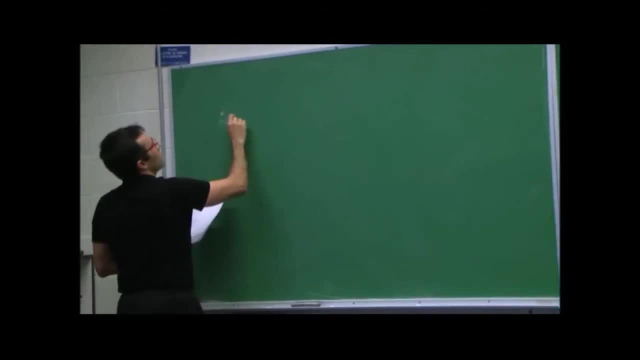 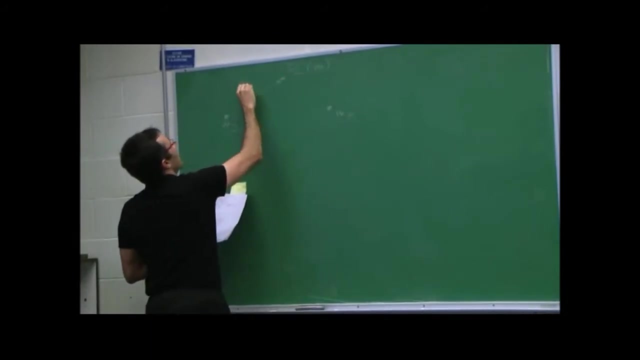 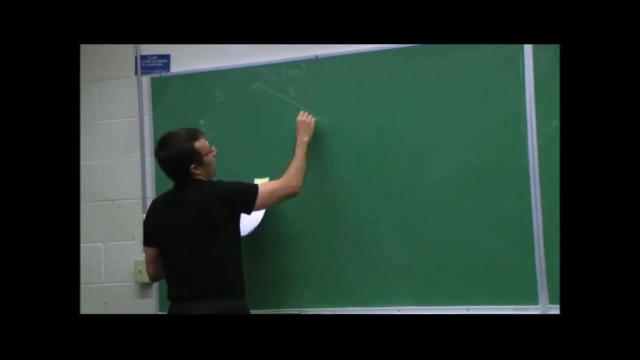 uh, sun, m? s is the sun. i have my planet somewhere else- m p, and i have my spacecraft somewhere else and i just say that this has a mass just m? um, and i'm going to call big r? s the vector. sun to space craft. uh, little r the vector, as we've done so far: planet, two spacecraft, this is the one we've. 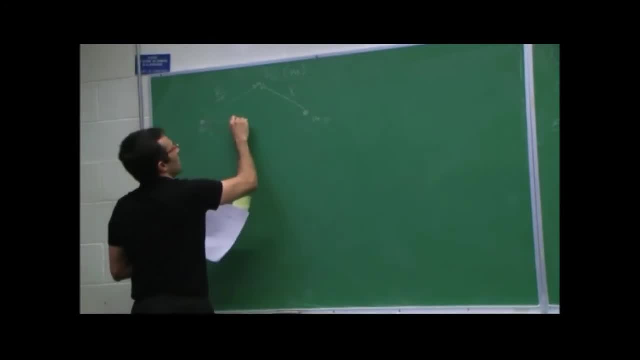 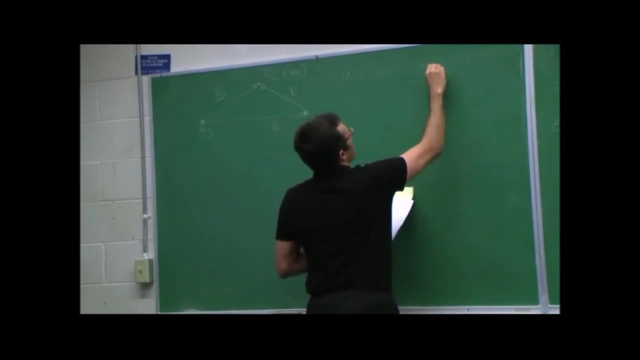 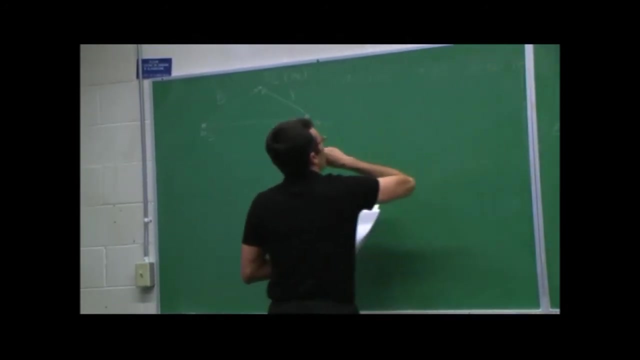 been dealing with for the entire semester. and then simply big r, the vector goes from sun to the planet. so i claim that i am inside this soi or sphere of influence, if the following happens. let's see how i call them. i call them perturbations and accelerations: yeah. 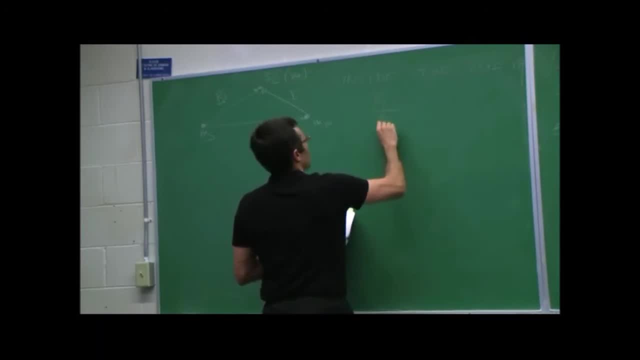 i'm going to explain what these are in a second. uh. ps over ap is less than p p over as, where by p i mean perturbation, they're, they're all accelerations here. but when i say p- i, i, i am looking at a perturbation. when i say a- i, i'm talking about a main acceleration. so what i'm. 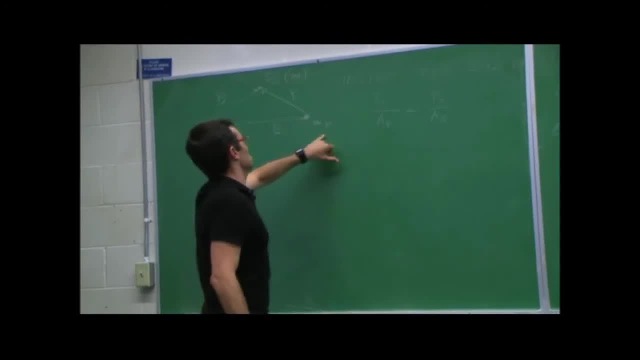 saying is that i am inside the sphere of influence of the planet p. if uh, the ratio between the acceleration on the spacecraft due to the sun over the acceleration due to the planet uh is less than uh, the perturbation due to the planet over the acceleration due to the sun does make sense. so 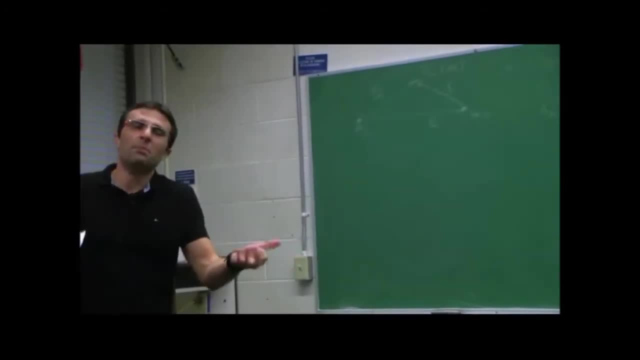 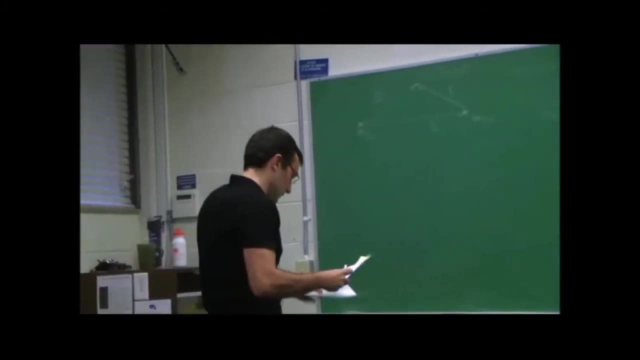 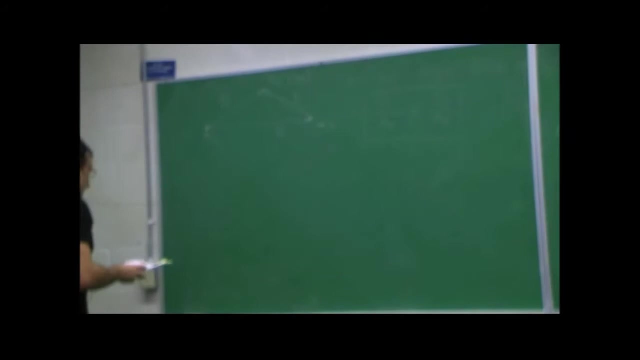 basically, you are inside the sphere of influence if, if the sun is a perturbation is less than what you experience because of the planet, and vice versa. you are outside of it if the sun takes over, which makes sense. uh, so that's exactly the expression that i'm going to base everything on at the end. uh, but 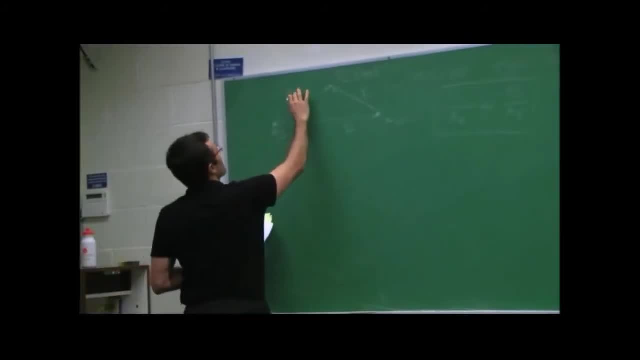 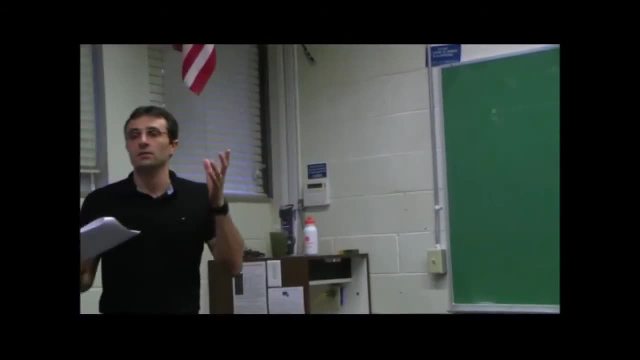 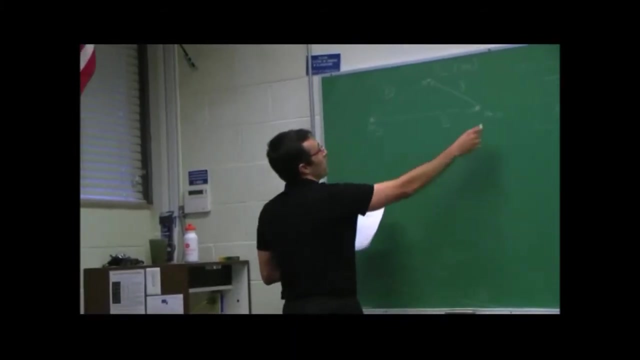 i need to compute- uh, the second time- derivatives basically of all these vectors here that are involved and do some simplifications. always keep in mind that the sun is a lot more massive than any planet in our solar system, which means, um, then, most likely, the sphere of influence of 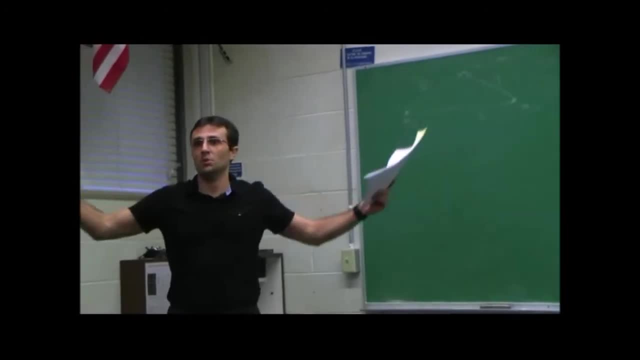 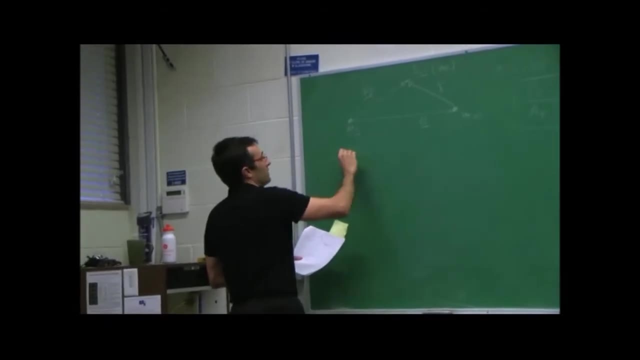 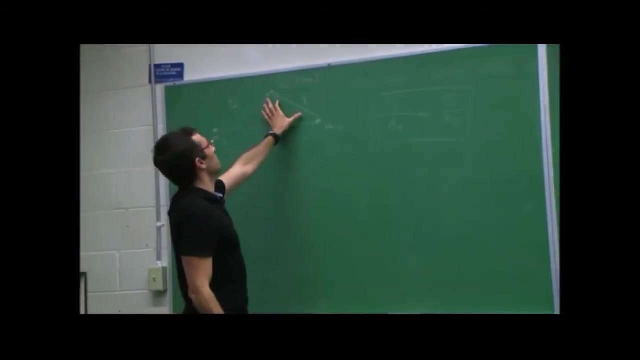 these planets will be tiny compared to the distances between planet and planet and planet and sun. so at some point i will make the approximation. not for now that, for example, r and rs are more or less the same thing that that this vector here. uh, to the spacecraft, if i am inside, 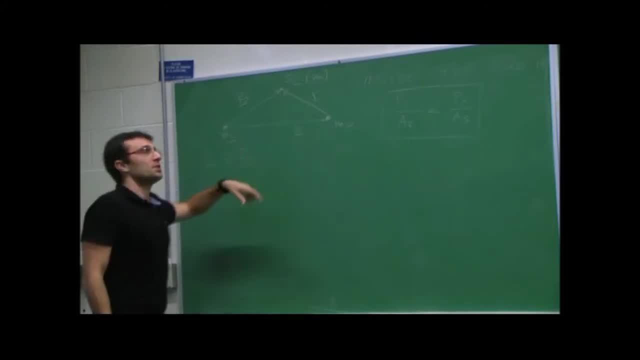 this fuel influence, of course. um, it's probably tiny. so you're sitting on the sun, you're looking at planet earth, for example, and a spacecraft that is orbiting earth and it's inside this influence. you're probably not going to even notice the size of these little. 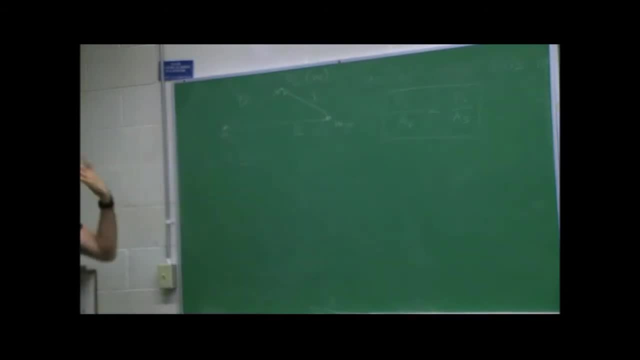 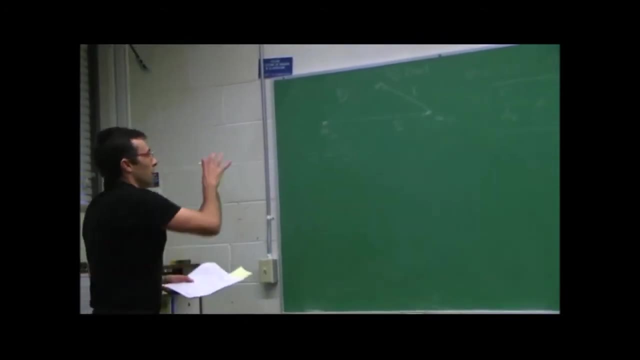 r, that is changing- make sense if it's inside the sphere. if it's traveling to another planet, then it's a different story, but then you're not inside the sphere influence anymore. so, but we'll use that as the main approximation. and then, of course, uh, it's obvious that the mass of the spacecraft is. 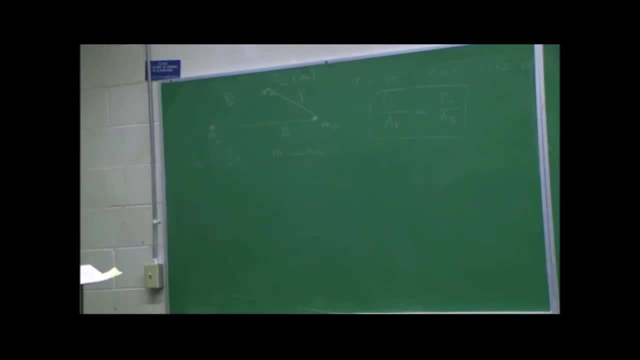 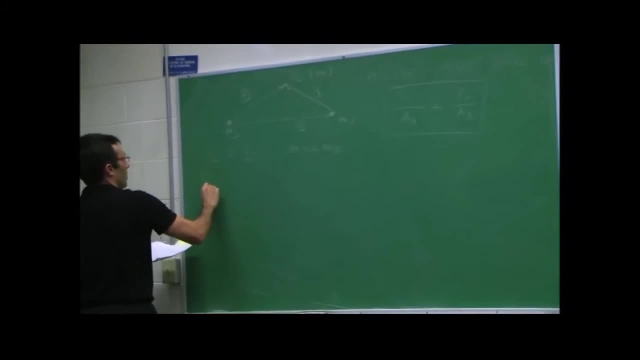 going to be definitely much smaller than the mass of the planet. we use that at some point- and even more with respect to the sun. but let's, uh, let's write a few forces here. so the force uh, on the satellite, due to the mass of the spacecraft, is going to be much smaller than the mass of the 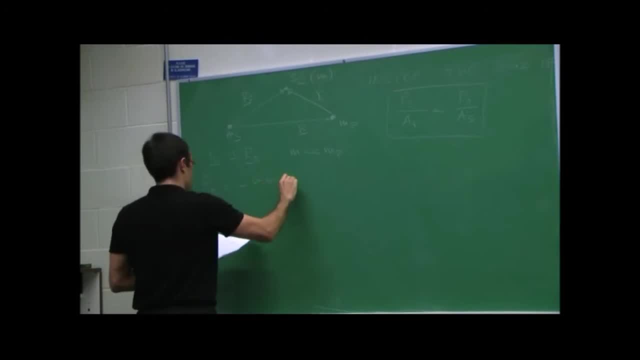 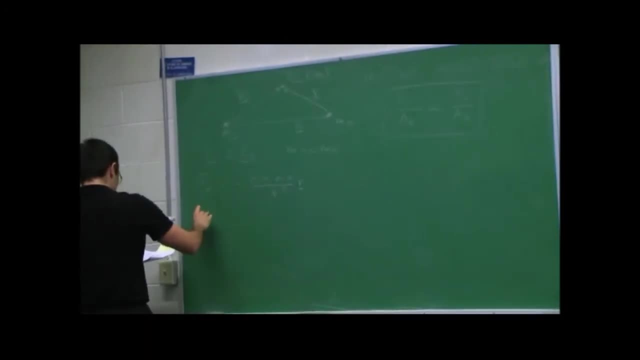 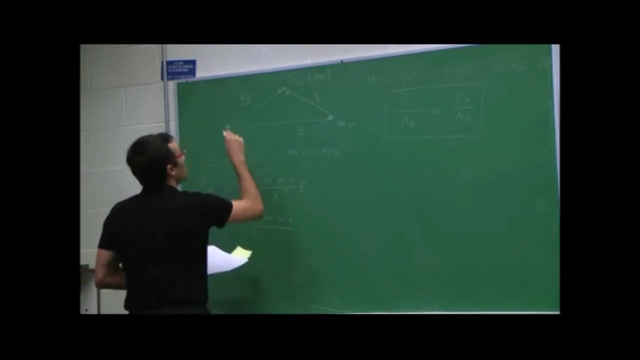 planet is, as we know, minus g m m of the planet. uh little r cubed r. that's the one we've been using all the time. the force on the satellite due to the sun is instead minus g m mass of the sun. what is that? that's rs cubed as well times rs as a vector, and finally, fsp. 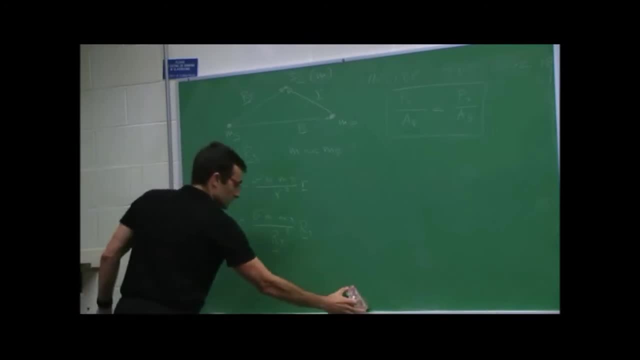 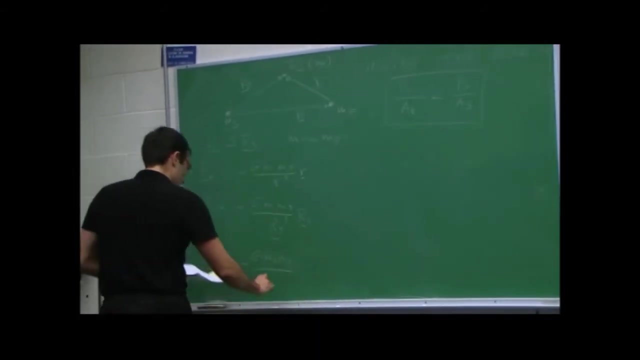 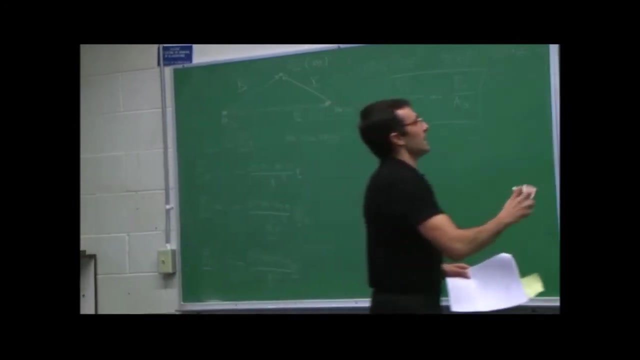 you'll be careful how much i bend, i'm sorry um. by by fsp i mean the force that the sun is exerting on the planet is minus g m of the planet, m of the sun over r cubed big r vector. okay, so let's start from rs. 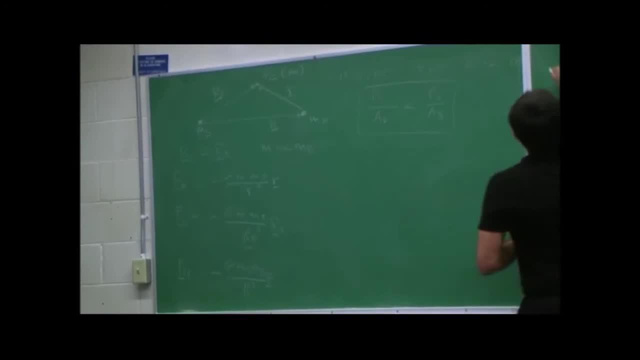 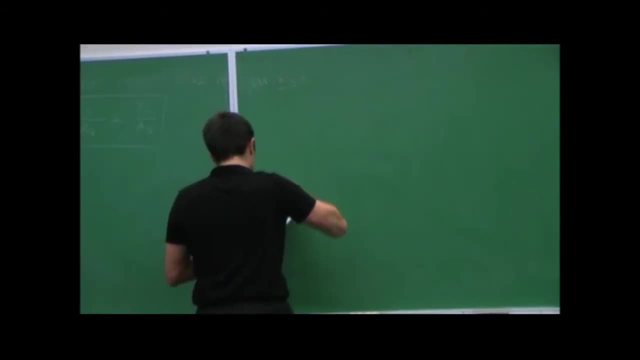 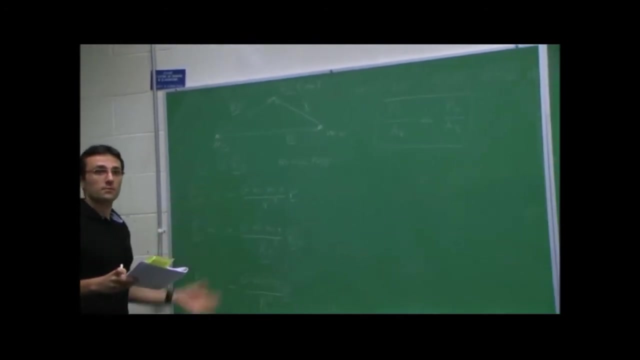 double dot. so, um, i know that m rs double dot is equal to what? what is this? now the sun for me becomes the inertial reference frame. probably, right? so this is all the forces acting on the spacecraft, which is the force acting on the spacecraft, which is the force acting on the? 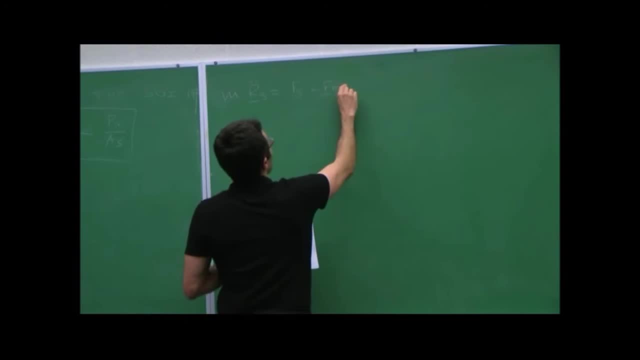 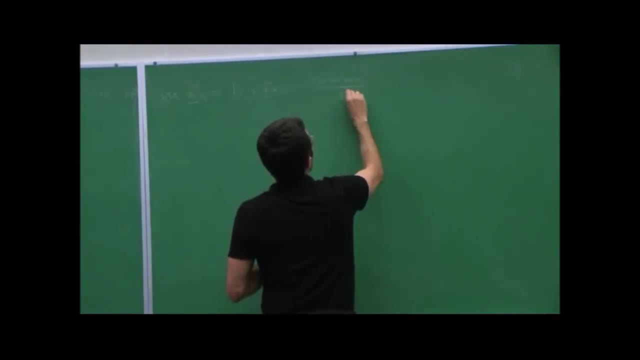 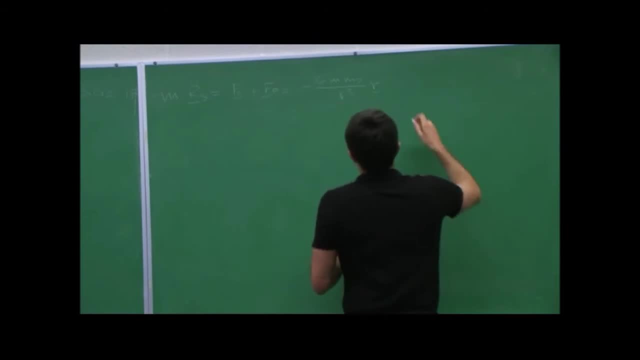 minus g m m of the planet. over r cubed times r times. r times r uh minus uh. minus uh. minus g m m of the sun- g m m of the sun. g m m of the sun. over rs cubed rs vector. over rs cubed rs vector. 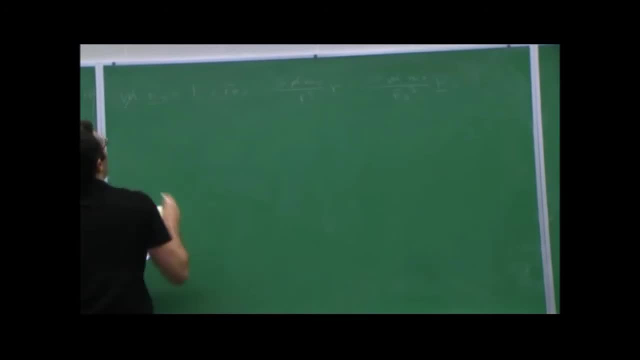 over rs cubed rs vector. so i can definitely, so i can definitely, so i can definitely. you know, simplify this, you know, simplify this, you know, simplify this. and just look at s double dot and just look at s double dot and just look at s double dot, which is given by these two terms. 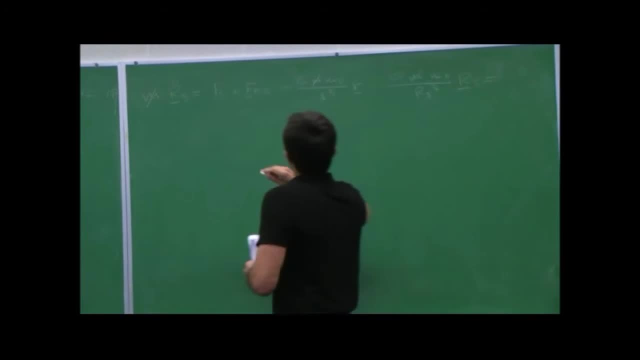 which is given by these two terms, which is given by these two terms: um, um, um. let's see, let's see, let's see. this is, this, is, this is so. this is going to be divided by m of. so this is going to be divided by m of. 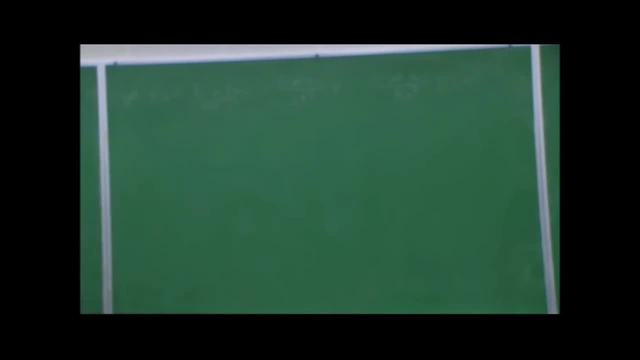 so this is going to be divided by m, of course, course, course, this is almost equal. if i, this is almost equal. if i, this is almost equal. if i start using these, start using these, start using these assumptions here, assumptions here, assumptions. here again, i am inside the sphere influence. 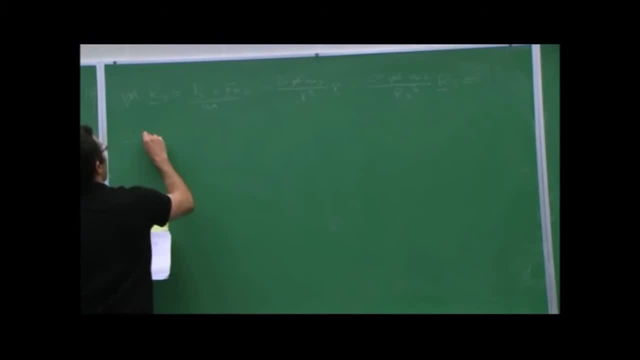 again, i am inside the sphere influence. again, i am inside the sphere influence. that's, that's. i want to compute the that's, that's. i want to compute the that's, that's. i want to compute the radius of the sphere influence. i have. radius of the sphere influence. i have. 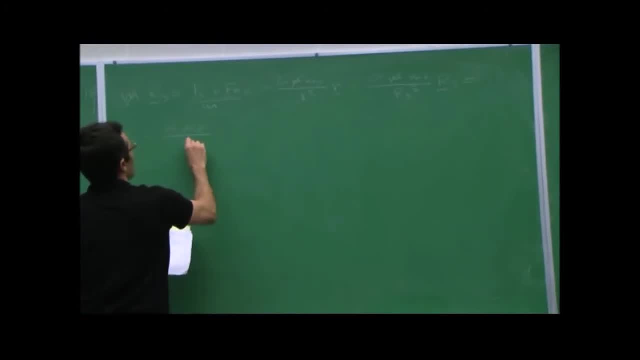 radius of the sphere influence. i have minus g minus g, minus g m of the planet, over m of the planet, over m of the planet, over r cubed r, r cubed r, r cubed r. minus g, minus g, minus g m. mass of the sun over 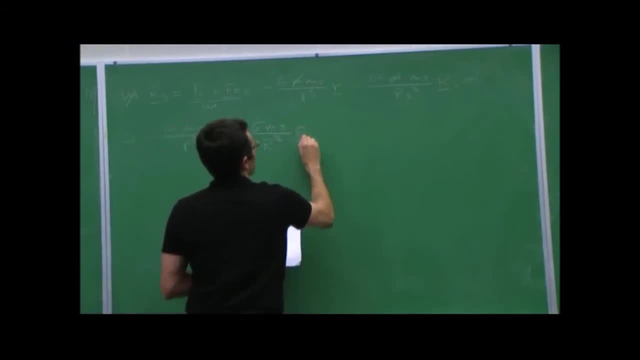 m mass of the sun over m mass of the sun over. so this just becomes r. so this just becomes r. so this just becomes r. right, if i assume that this is true, if i assume that this is true, if i assume that this is true, okay, okay. 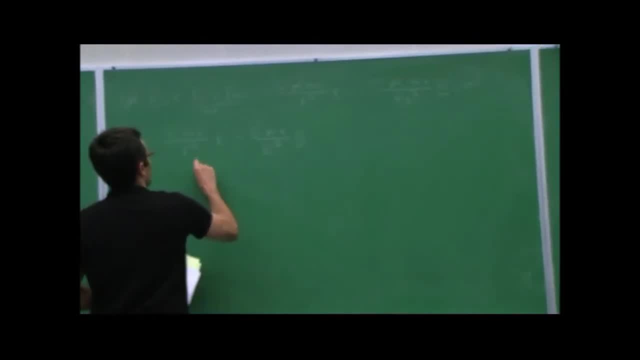 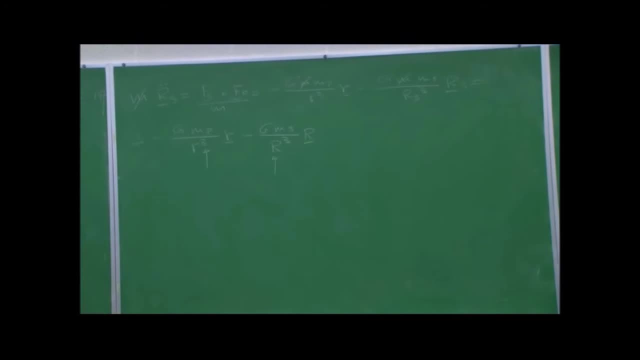 okay, and uh, and uh and uh, i'm going to call this, i'm going to call this, i'm going to call this and these and these and these. what I need to find something to plug into this expression, because that is the one that will give me. 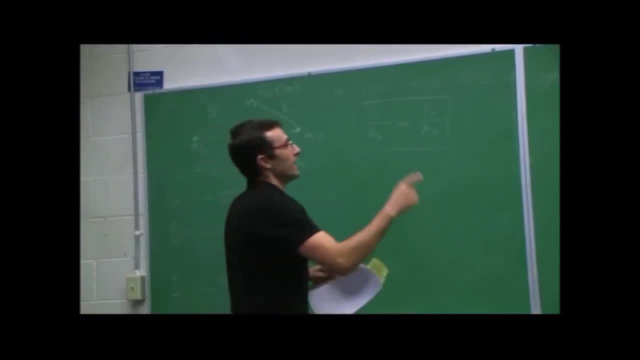 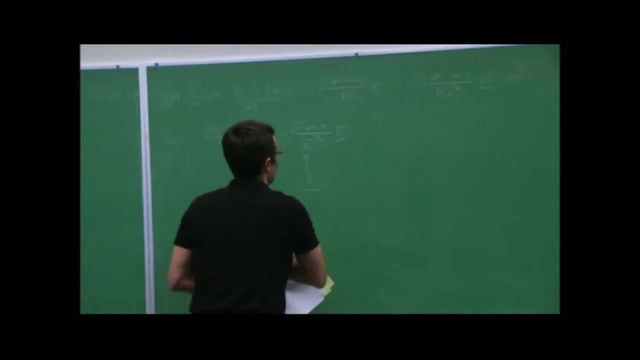 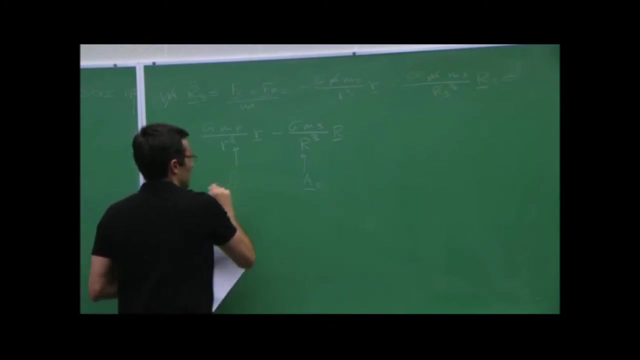 my sphere influence radius eventually. so I have two of these elements here. which ones? what do you think? this is more or less the acceleration due to the sun on the spacecraft, and this is, in this case, I call it the perturbation due to the planet on the spacecraft. 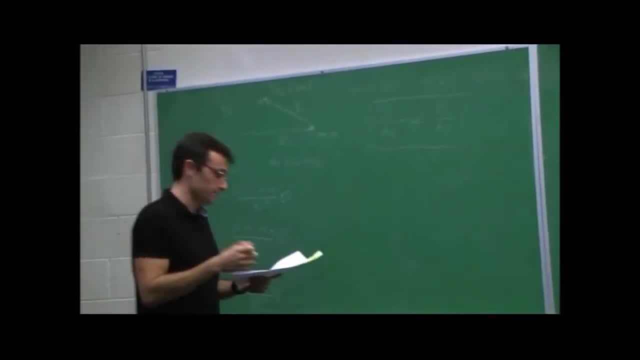 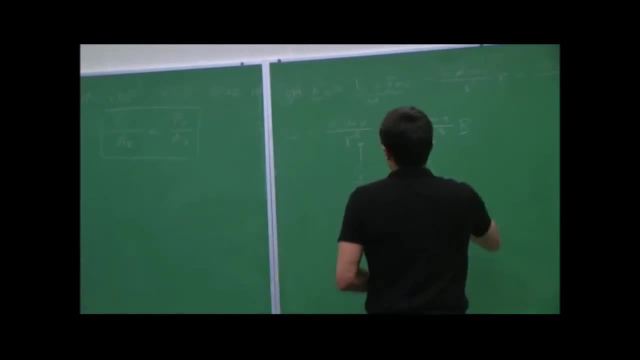 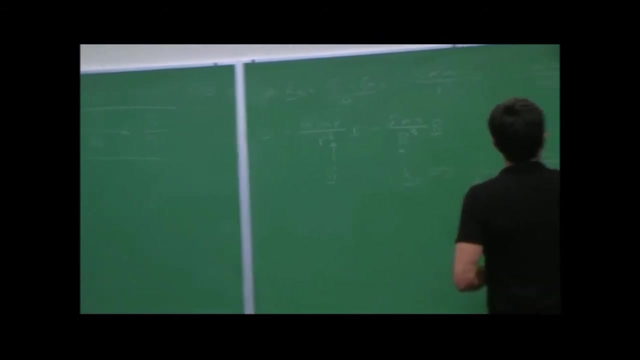 ok, and so I can do the P P over A S and I'm going to copy it there in a second. so I'm just looking at the norms: P P over A S. let's see, is G and planet over little R, cubed R which divides. 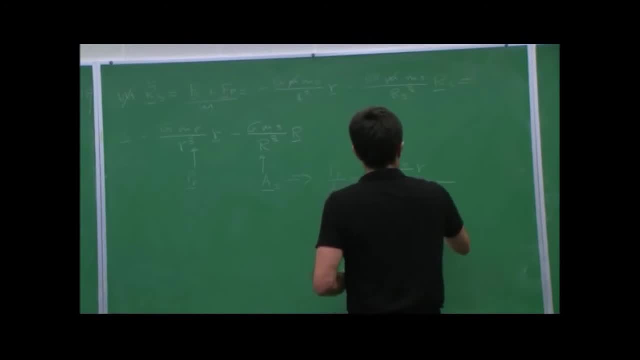 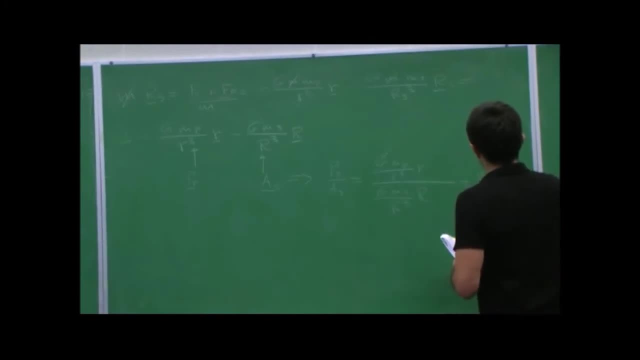 G M sun over R cubed big R. simplify a few things. here you are left with M planet over M sun, big R over little R squared, so I'm going to actually substitute that in this expression right here. let's see: M P over M S, big R over little r. 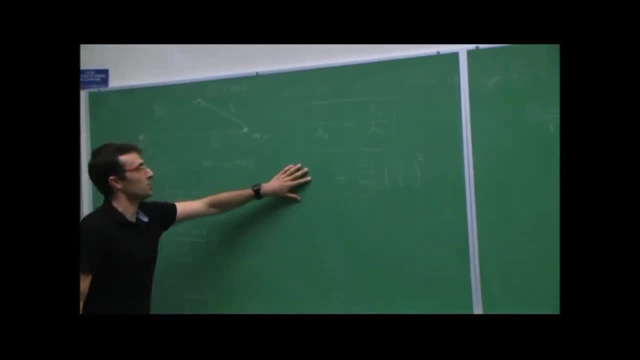 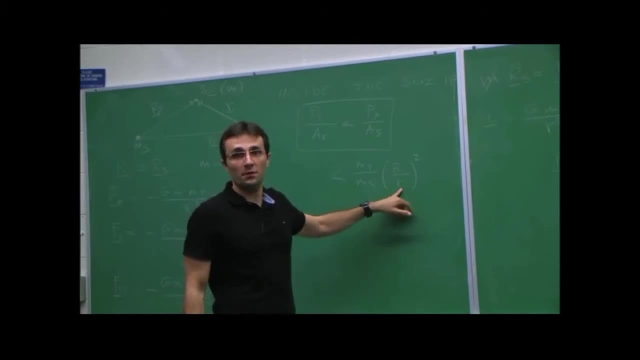 squared. so eventually, from this expression I need to substitute something here. I will solve for little r and that will be my radius of the sphere of influence. ok, and you can start seeing that all I want to see appearing here are masses of the planet and sun, of course. 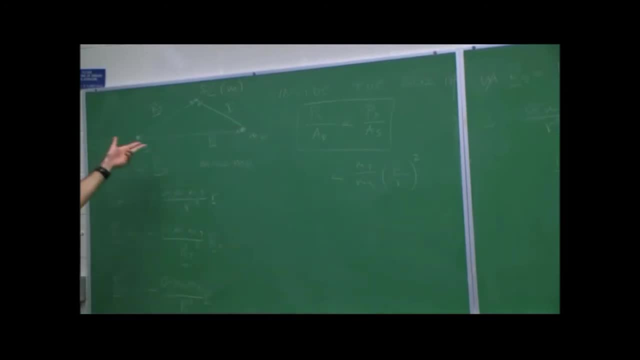 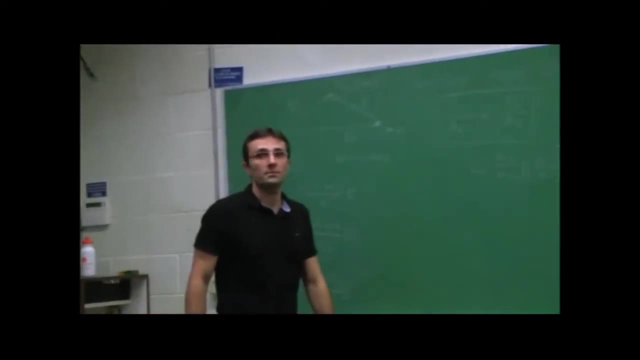 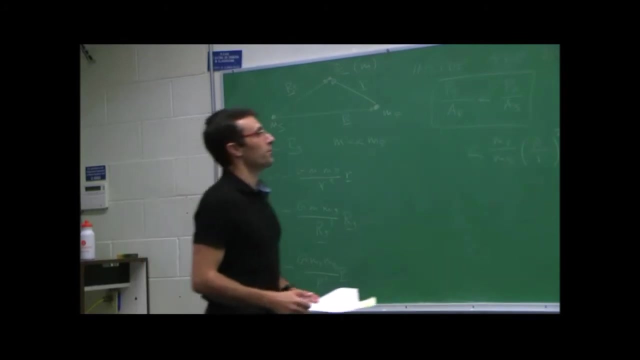 and the distance between the planet and the sun, which makes sense, because probably if you're closer to the sun, your sphere of influence is going to suffer, kind of become smaller. it's easier to get attracted by the sun, right? ok, so that is the first piece, or second piece, of this inequality. 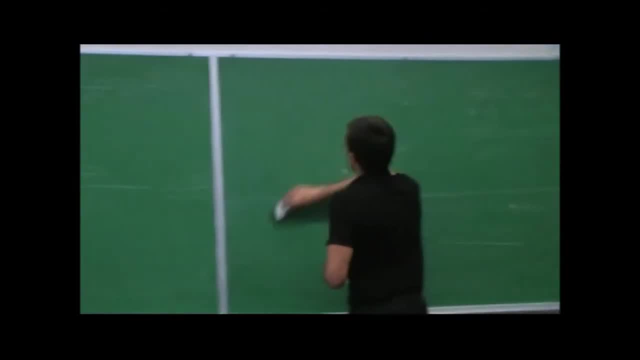 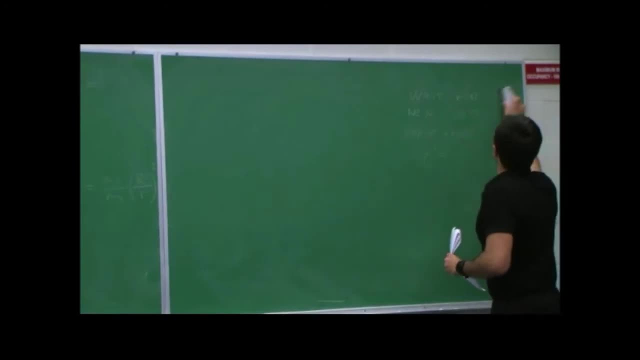 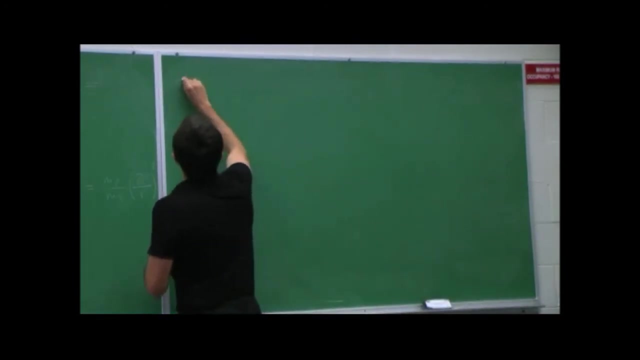 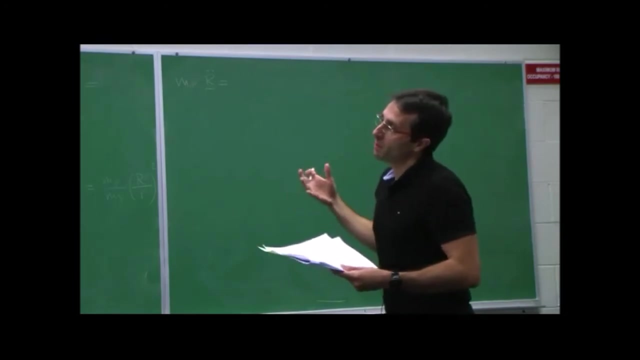 and then we'll do something else. let's see what do we do. we need to look at the planet for a second. M P? r double dot is equal to. in principle, the planet is attracted by the sun and the spacecraft. of course, what the spacecraft does to the planet is kind of ridiculous. 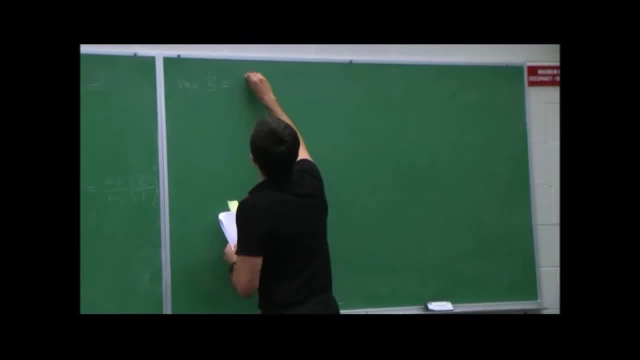 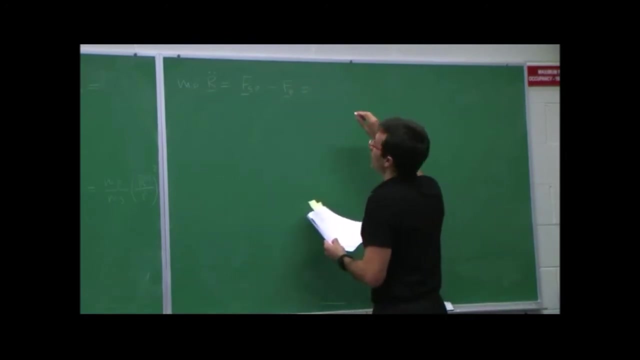 but we're going to have it there for a second. so this is actually the fsp that I wrote down there, minus actually the f. what did I call it fp? so this is, let's see g. what is fsp minus gms, mp over? 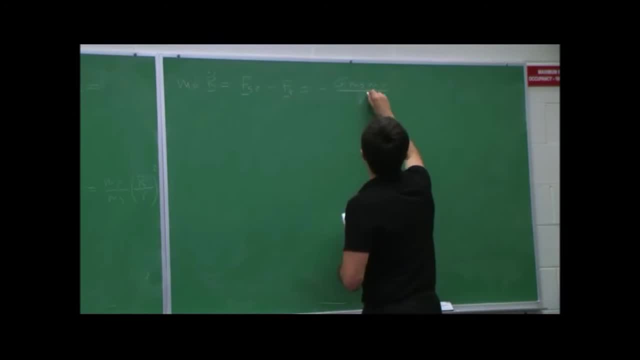 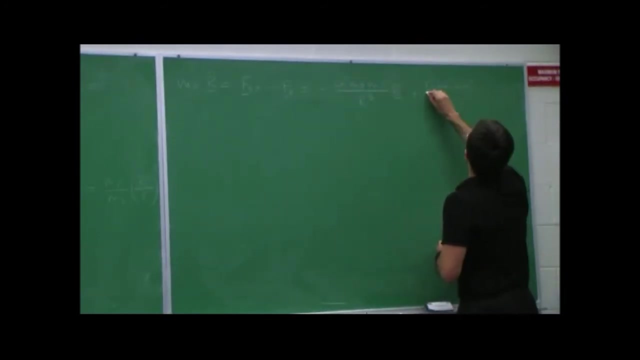 that's r, big r cubed r. and then I have minus, minus, right, yeah, plus gm m of the planet, little r cubed r. alright, I'm going to do the same I did with the other equation: divide by the mass, divide by the mass. 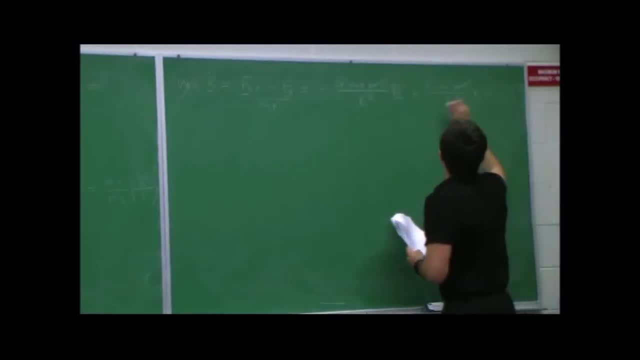 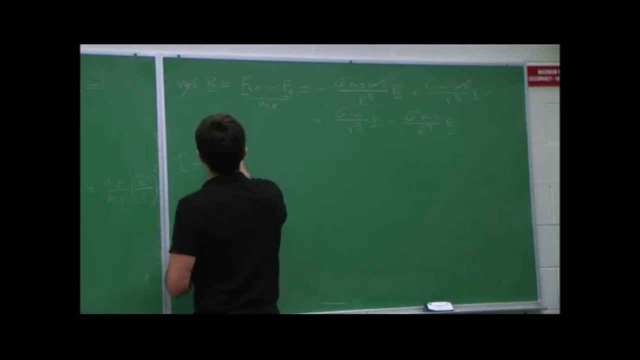 divide by the mass, and that's what I have: gm over r cubed. little r minus gms big r cubed r. that's fine. now we're going to put together the little r double dot factor, which is big r double dot s minus big r double dot. 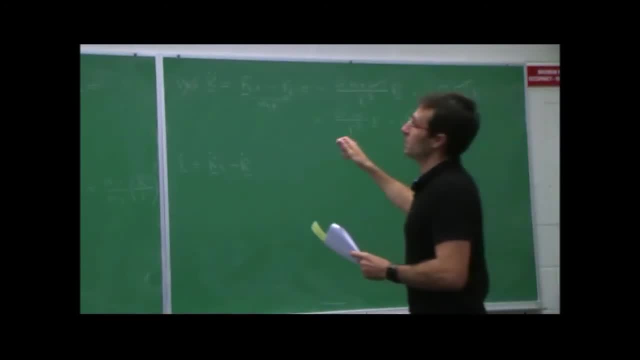 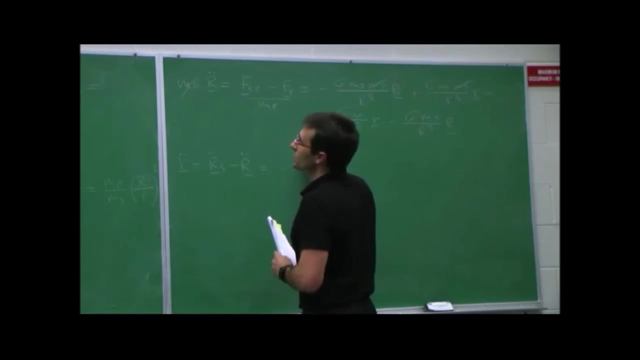 which I have. I have both of them. I have this expression here before I simplified it, and then I have this expression here, so I can just subtract the two. let's just write them as they are for a second. I have minus g. mass of the planet, gm. 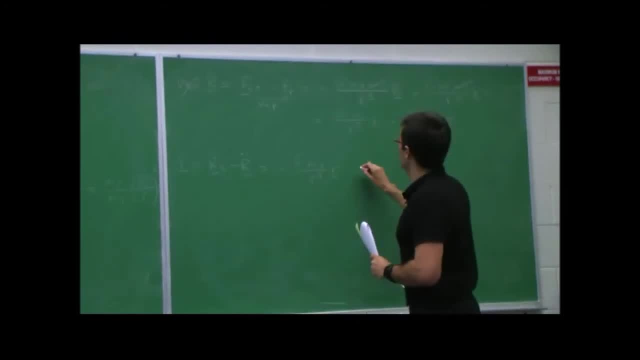 over r cubed r with a little r minus g ms. I'm going to keep using rs for a second and then I will simplify at the end. so this is rs double dot minus all this: minus gm over r cubed r and plus gms over r cubed. 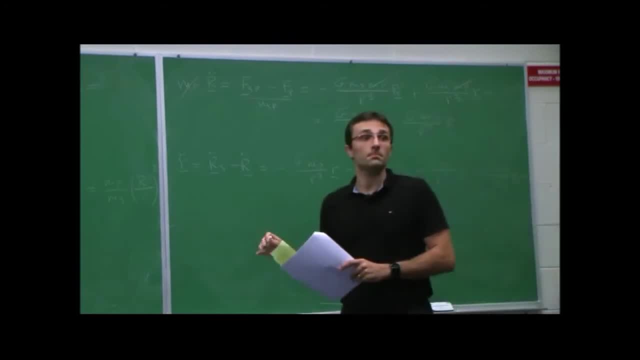 r. ok. ok, so this makes sense. yes, so I have a question: the right: if you cancel the ms, how do you cancel that? because you divide it by m. yeah, no, it's not cancelled, thank you, thank you. no, I think there is hold on, hold on, hold on. 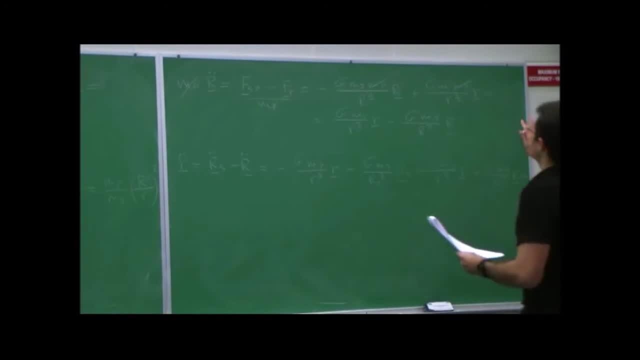 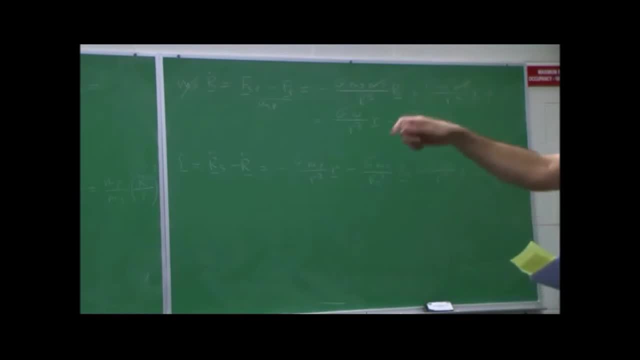 right, if it's correct, that is the force that the planet experiences because of the sun. so that has to be mass of the planet and mass of the sun, and so we have them there, and when I simplify with the mass of the planet, that becomes an MS and that's. 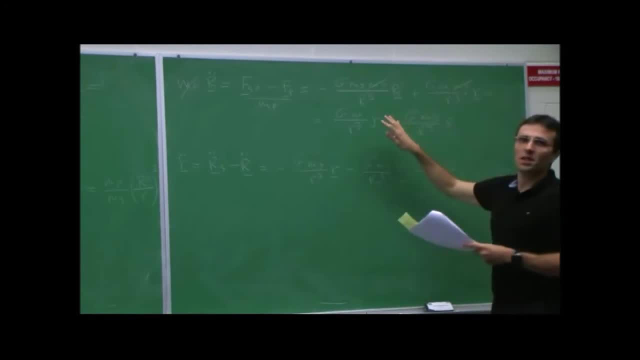 right here and this is spacecraft, so it should be okay, right? yeah, I mean that will pretty much disappear at some point, but that the second force- once I divide by the mass, it's an acceleration- is this one here and it's what the planet experiences because of the spacecraft. 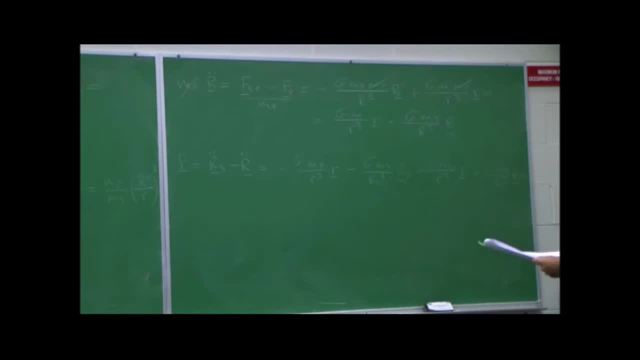 I will get rid of it, but yeah, anything else. so you don't need that S now. I do not. yes, thank you. okay. so let's collect a few things together here. I like this one and this one. they can go together somehow and this should become. let's see what I have here. 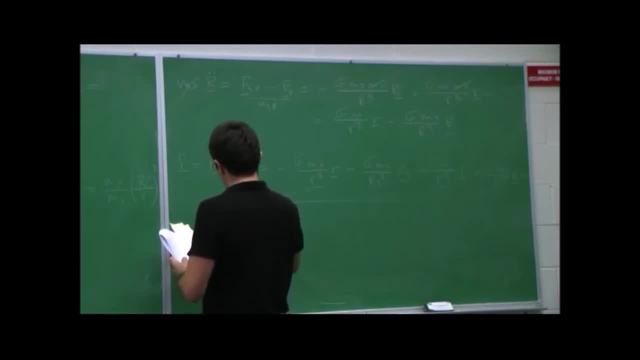 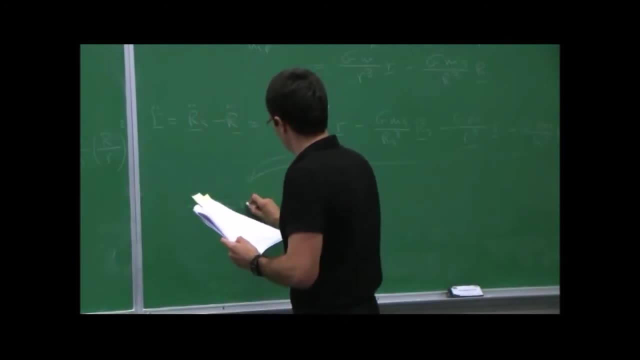 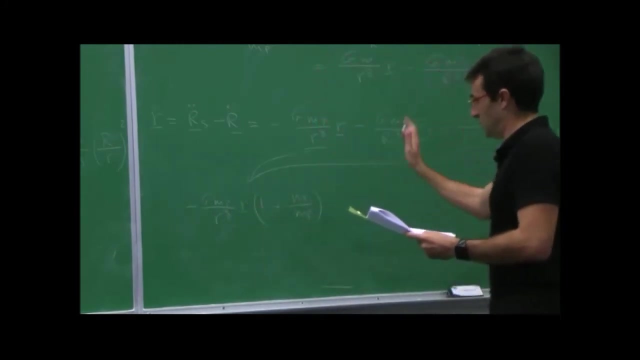 yeah, I have a minus G mass of the planet over R. cubed little r. that multiplies one plus mass of the spacecraft over mass of the planet. as you can imagine, this will just disappear because mp is much bigger than m and then I have minus. I like these two together because they have GMS. 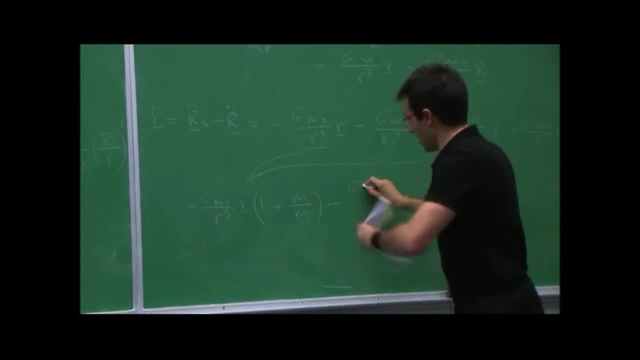 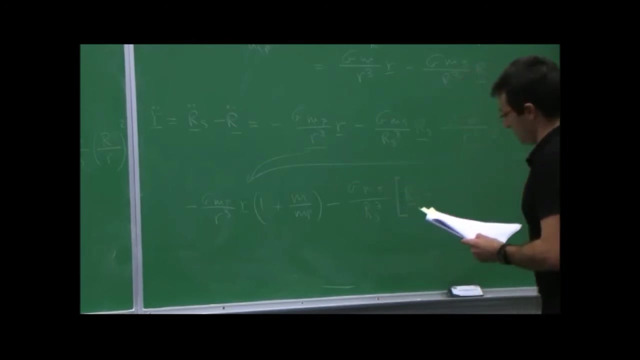 G MS over. let's see what we can do. we can do different things, but let's collect these RS cubed. that multiplies RS minus. let's make it a square bracket here. simply RS over R cubed over R cubed, right, these two terms make sense. 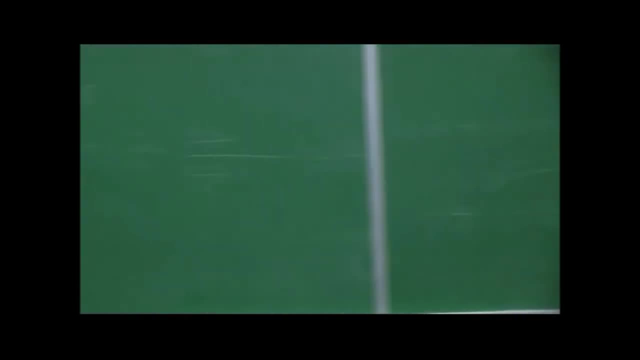 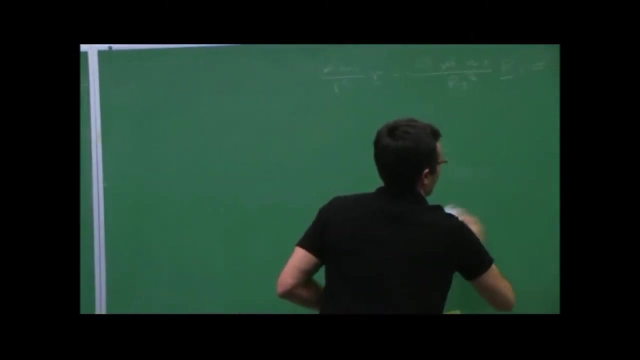 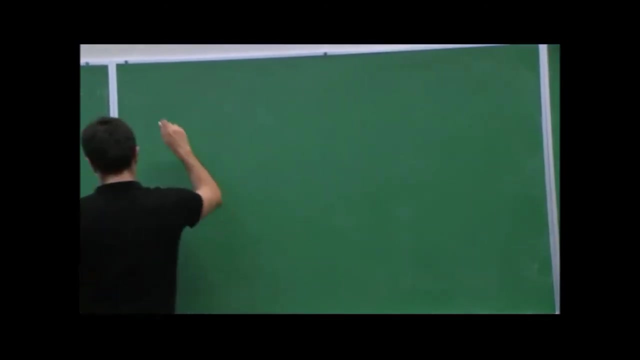 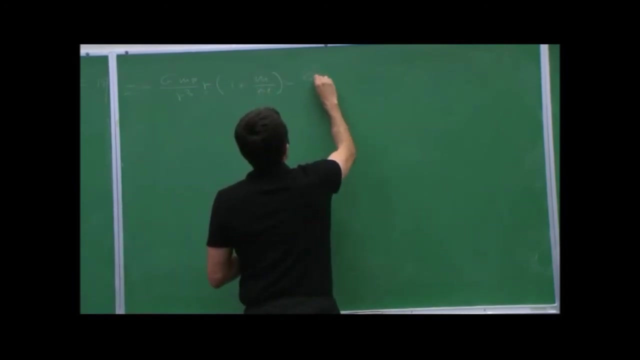 I'm going to move all the way down here, not here, okay. so let's manipulate that a little more. I have minus G mass of the planet over little r cubed. R one plus m over mp. that has not changed. but then I have GMS over RS cubed. 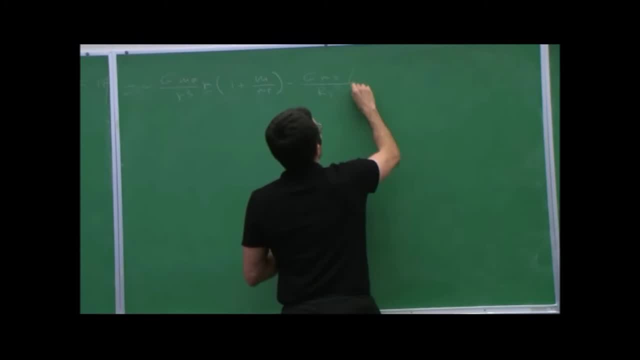 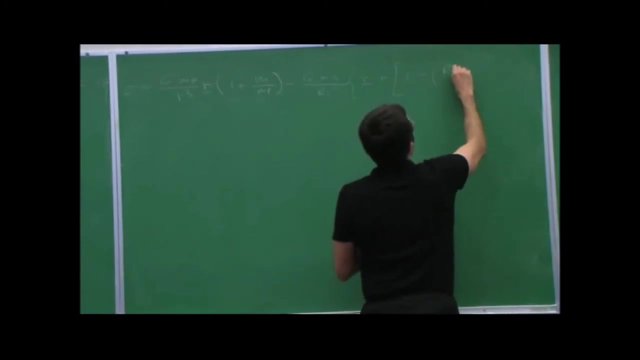 I have a few more parenthesis here so you can add and subtract big R, so you can make little r appear here. but then you have this correction: one minus one minus RS over R cubed. that multiplies big R makes sense. what I've done here, little r again is: 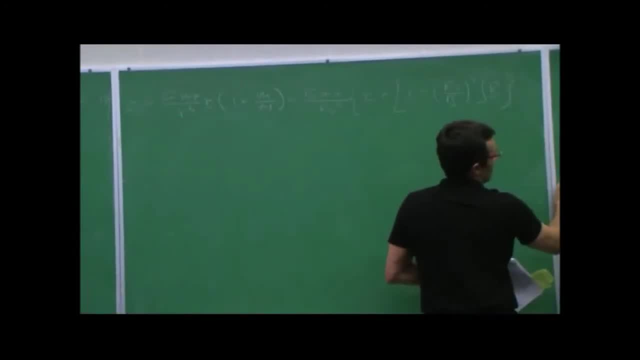 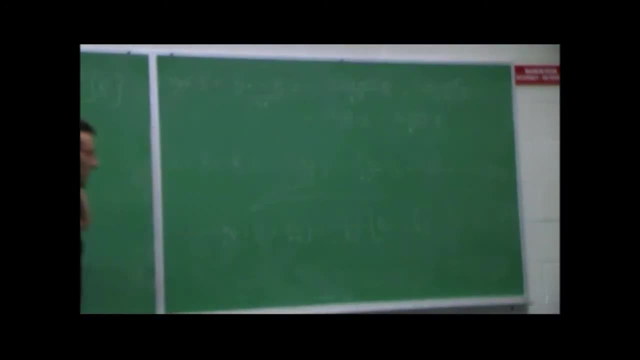 well, aside from the double dots, little r is RS minus R. so if, inside these parenthesis, I subtract a big R, I have to add back a big R. so this is what comes out of subtracting, and this is the additional big R. this is what comes out of subtracting, and this is the additional big R. 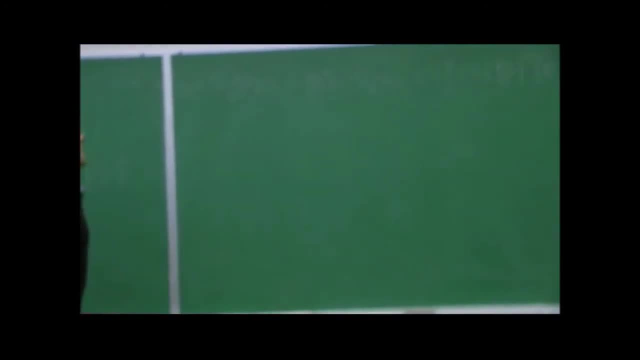 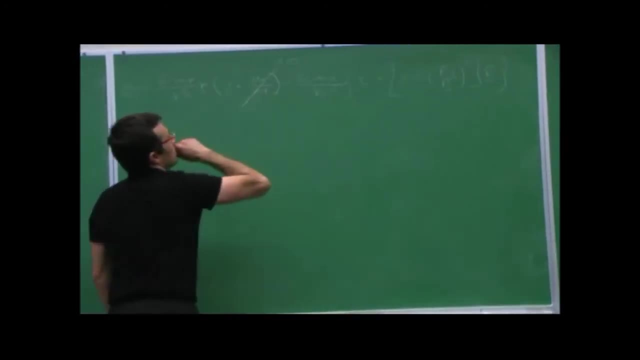 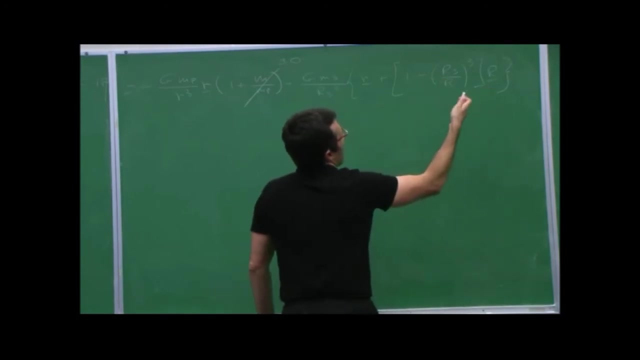 this is what comes out of subtracting and this is the additional big R. now I can make my simplifications right there. this goes away. this is about zero, pretty much. and if RS and R, this is not a vector, if RS and R are comparable, because I'm definitely inside the sphere of influence. 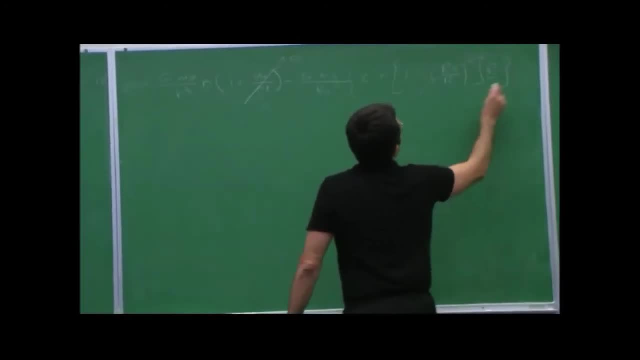 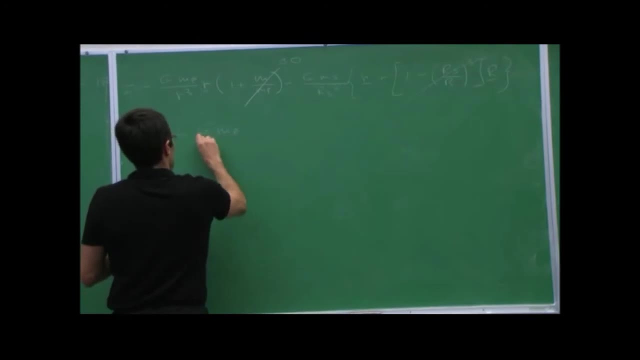 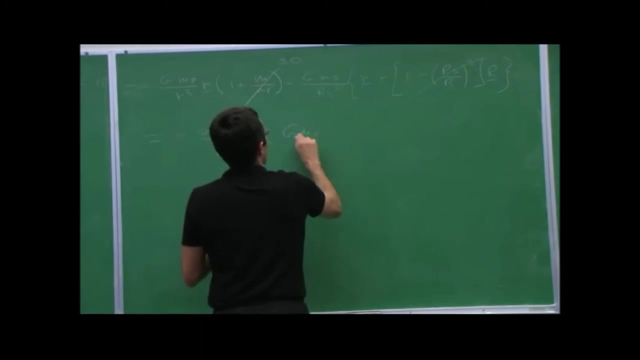 that's what I'm looking for. this becomes a one. this goes away. now I should see something that looks like: minus g m p over little r cubed times r vector minus g m s. again. at this point, RS and R, the two capital Rs, are the same thing. 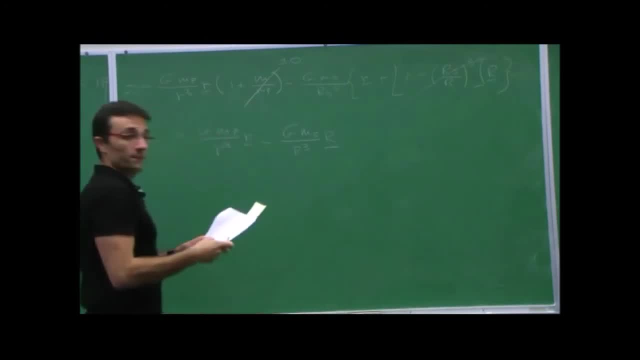 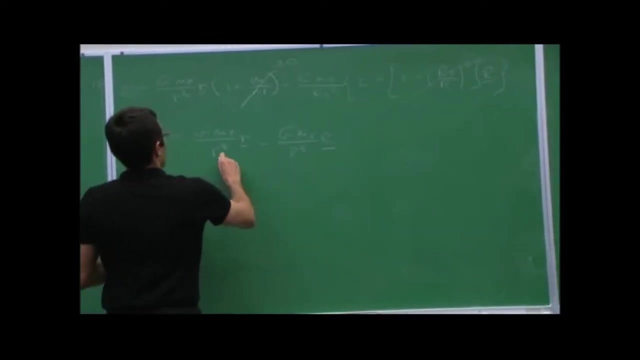 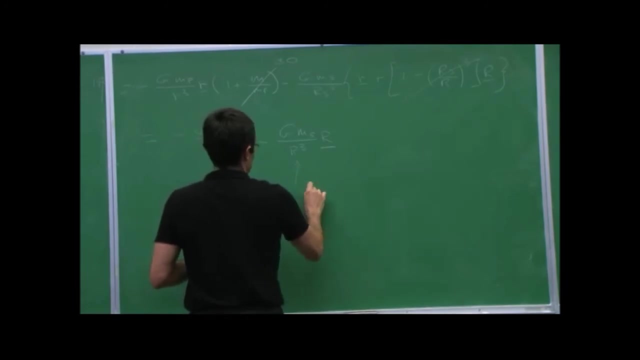 so I have big R, cubed R. that's a little bit of algebra. I'm going to call these two pieces well, this is now the acceleration due to the planet that I need there and this is the perturbation due to the sun. yes, excuse me, why is that the big R vector? 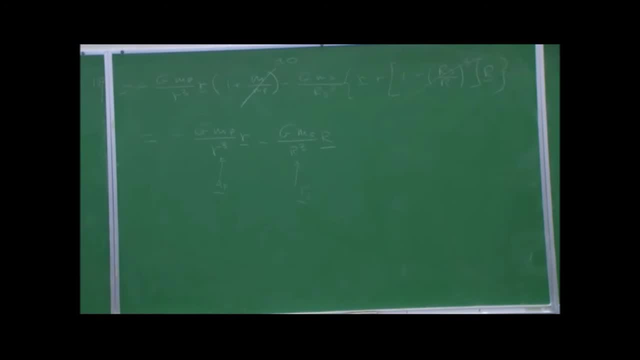 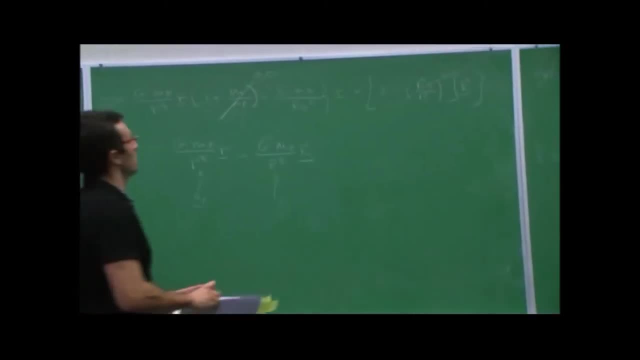 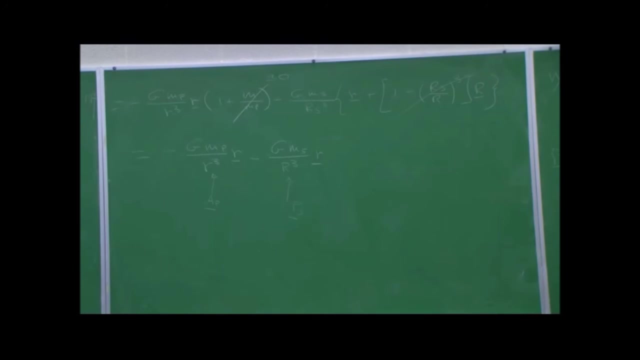 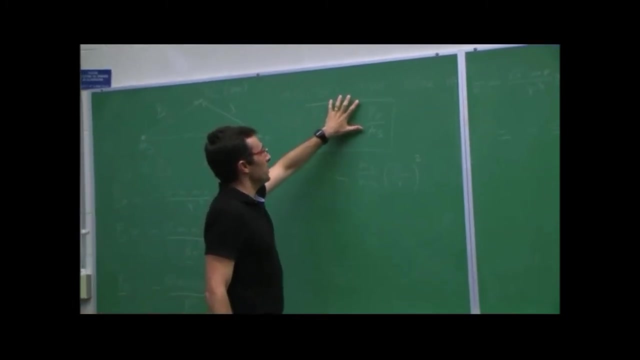 instead of the little r vector right there. I use the two assumptions, but it's the little r vector up there. see it is. thank you, that's right. so is the line of thinking clear. this is the starting point and that's why I started from this. this first ratio gave me 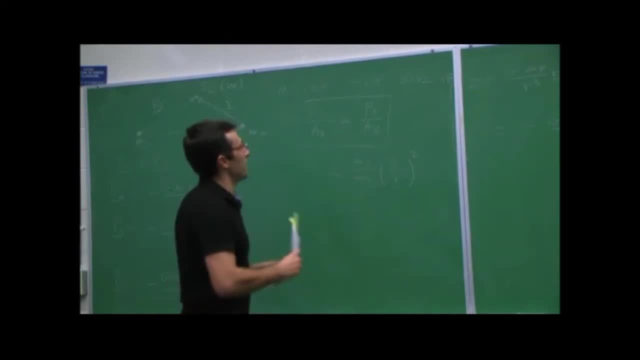 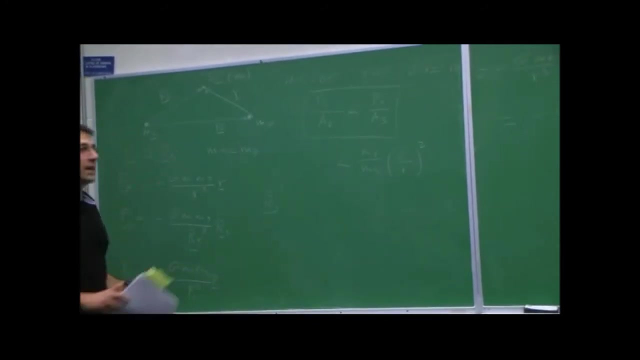 perturbation due to planet over acceleration due to the sun. that's why, to compute this one, I started from looking at this. acceleration, like my spacecraft, is mainly orbiting because of the sun, and the earth, or the planet, is a perturbation, something that is annoying me, right. 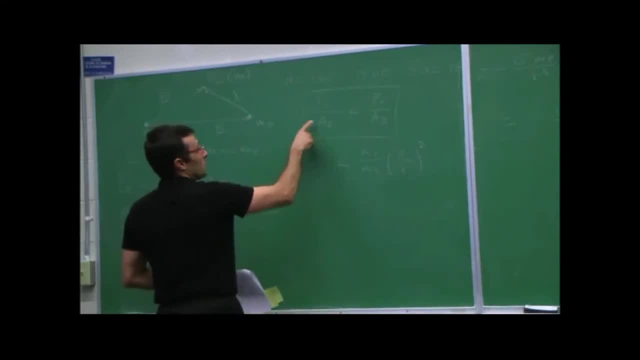 so that's how I get this ratio, while this other one is the opposite. that's why I started from this vector here, which is the usual one we use in astrodynamics for orbiting around the planet. make sense? ok? well, I have to compute this ratio. 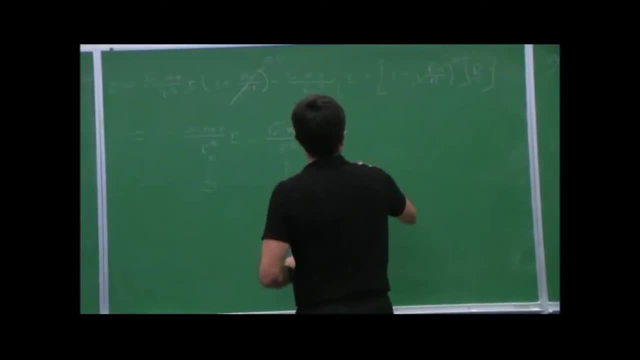 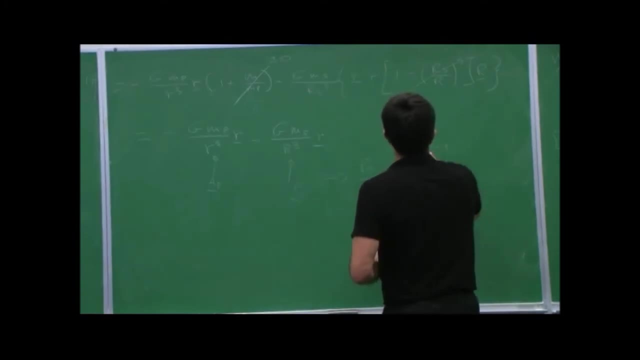 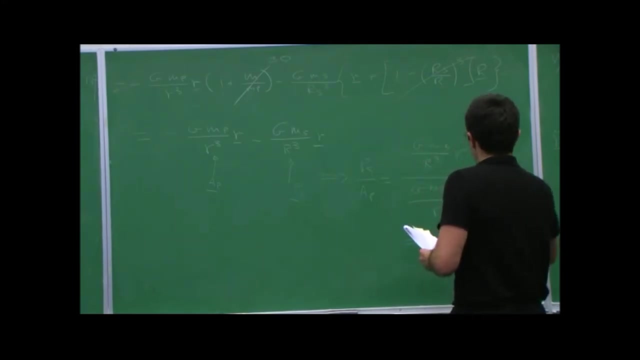 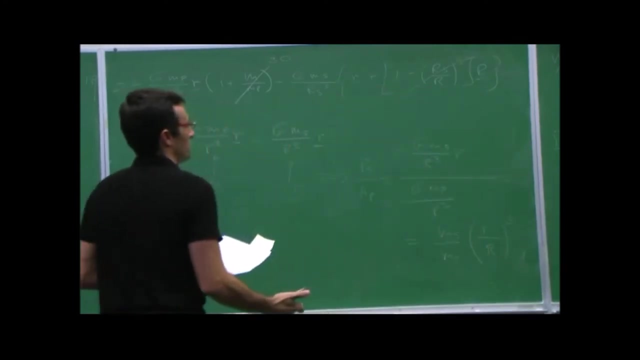 now. so what is ps over ap? let's see what we get: ps g ms over r. cubed r over g m planet over simply r squared, which in the end gives you ms over m planet. little r over big r. this time is cubed. now, if you're asking yourself, 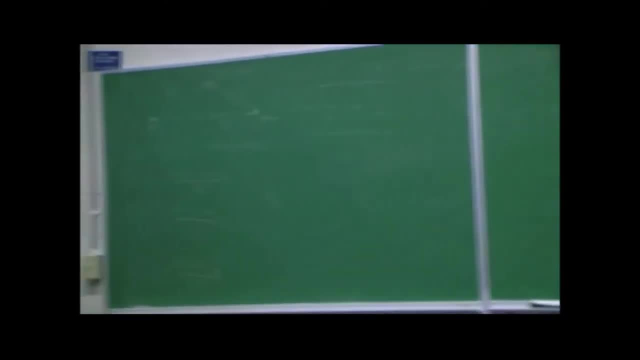 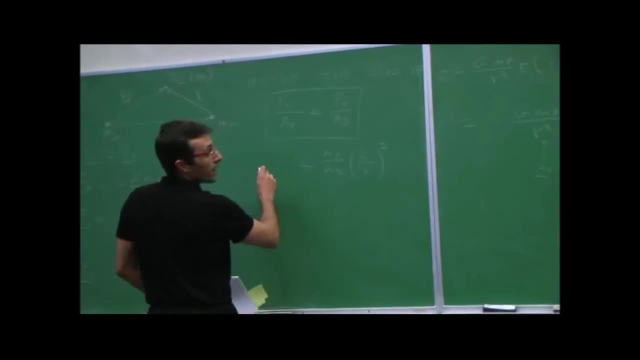 this is squared, that's cubed, that's fine, that's ratio of two distances. these ratios are dimensionless, so it still works. so that's what I want to substitute in here: ms over mp. little r over big r, r cubed. and now I have my inequality. 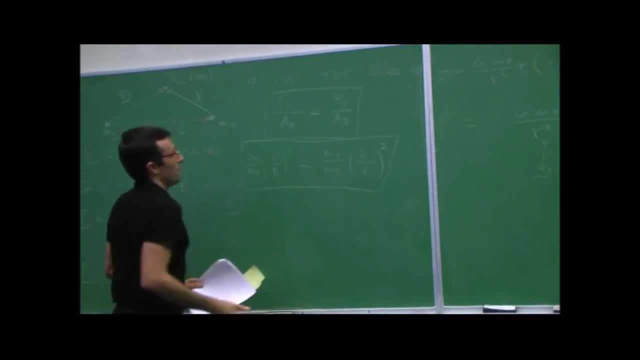 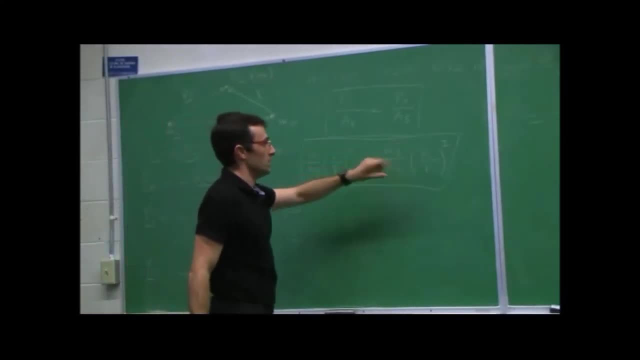 that I'm going to solve in terms of the little r, because that would be my sphere of influence around this object. that satisfies this inequality. if this inequality doesn't hold anymore, then I say that I'm outside the sphere of influence. so that's an additional step. 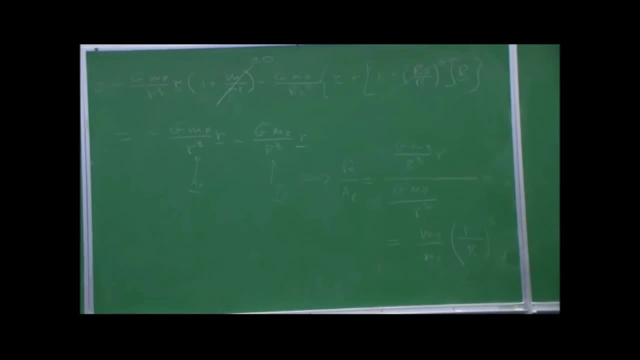 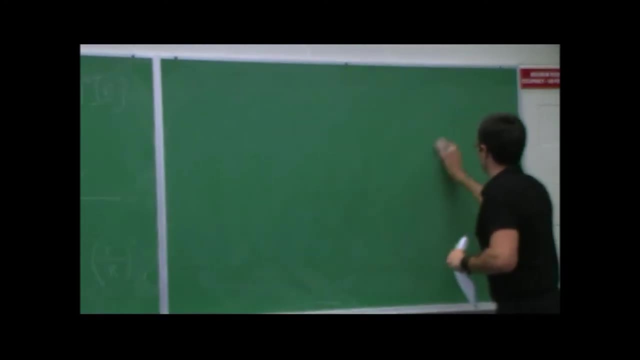 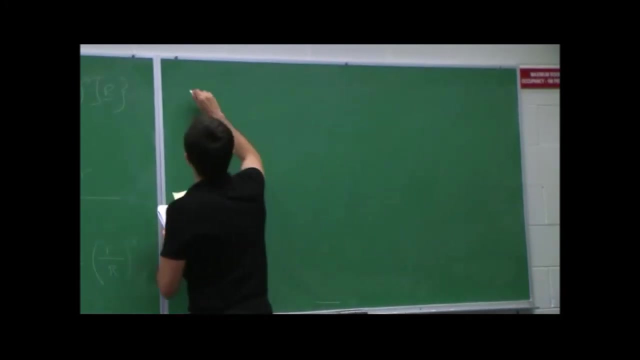 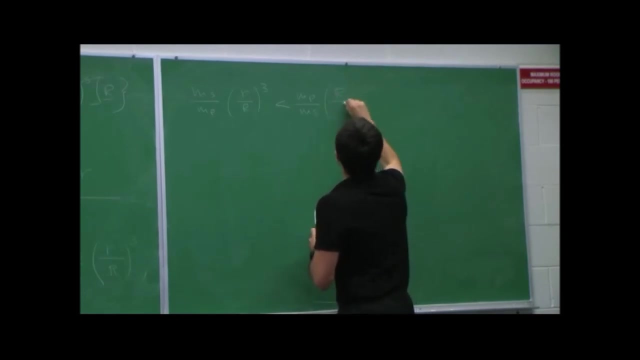 which we can do down here. alright. so I have ms over mp, little r over big r. cubed has to be less than mp over ms, big r over little r squared. so in the end I have this expression on the left: little r over big r. to the fifth. 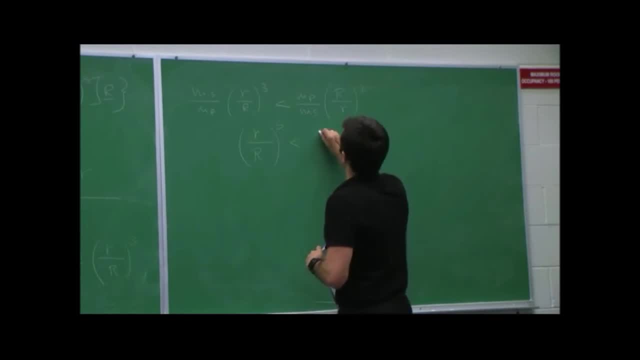 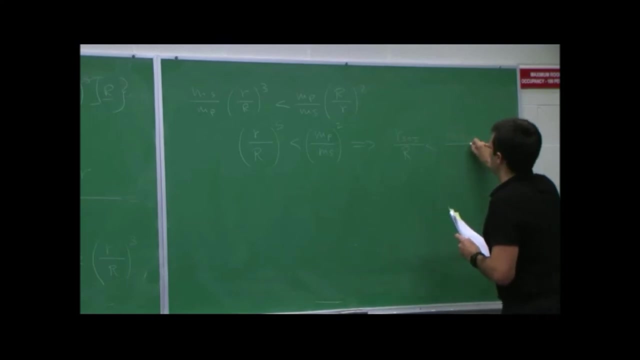 has to be less than msun. I'm sorry, mplanet over msun squared yup, and so, if you want, you can say: the radius of the sphere of influence is less than mp over ms to the two over five, and that's the end of the story. 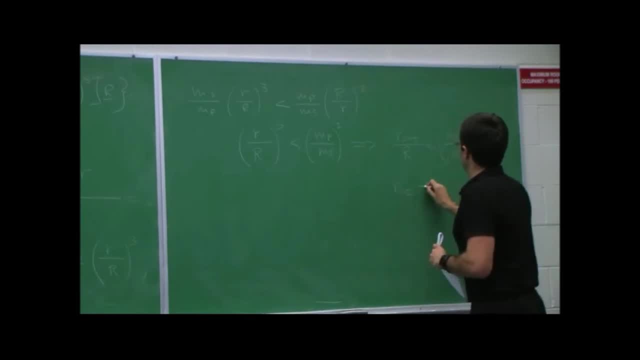 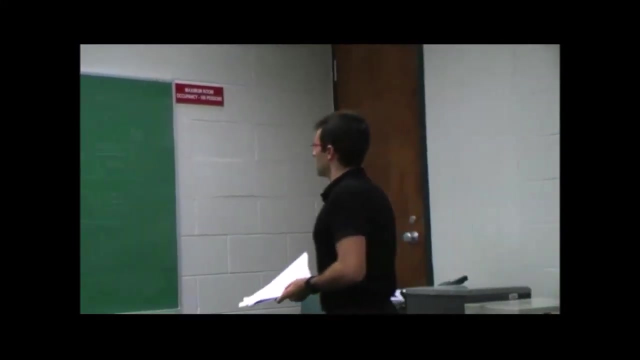 or, if you want to multiply it times r, but that's how you get it. so so if you're given a planet, you know its mass, you know more or less the radius of the orbit around the sun. you know the mass of the sun, you get the influence. 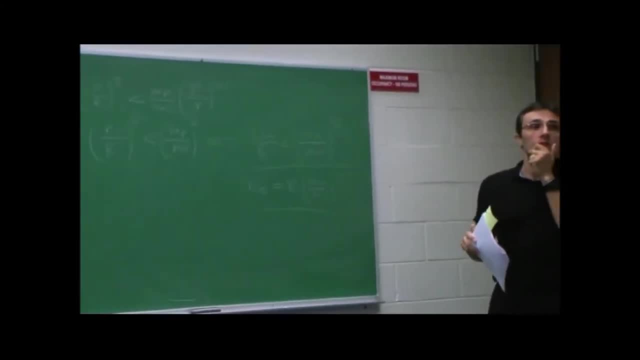 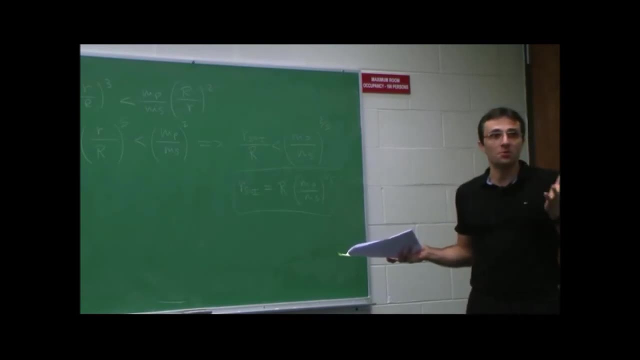 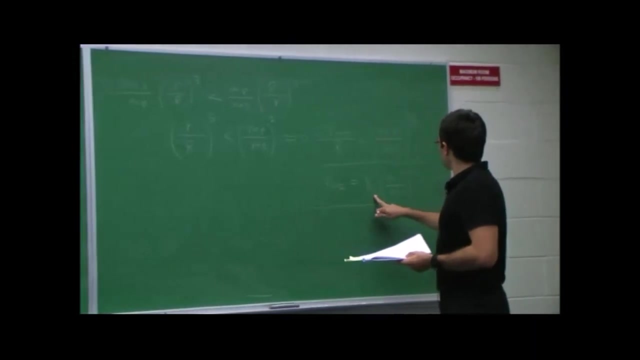 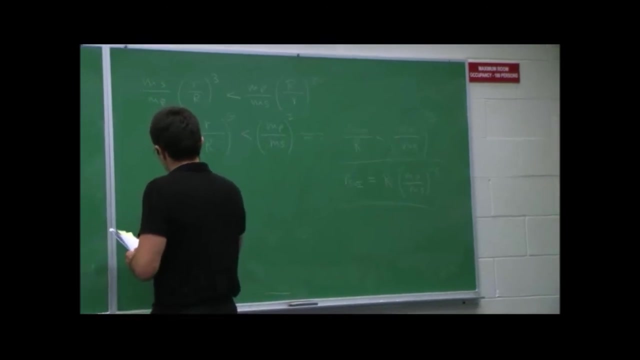 um questions. is the procedure logical? makes sense? again, this is only an approximation. of course, you are subject to everything at the same time, but it's a. it's a matter of how much. what is dominating now, as an example? the of the earth. I'm not going to give it to you. 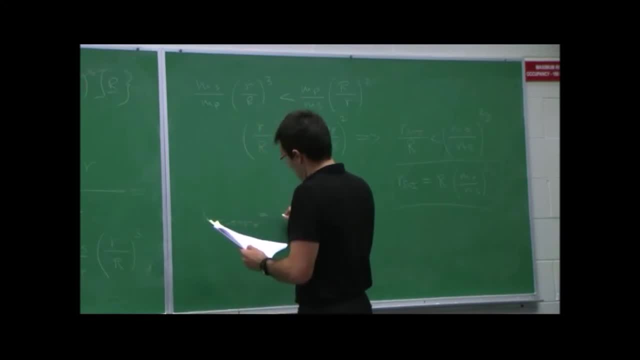 number I'll just give it in perspective of the radius of the planet is 145 times more or less the average radius of the Earth times. This was 6,000 plus kilometers, So the sphere influence of the planet is 140 times. 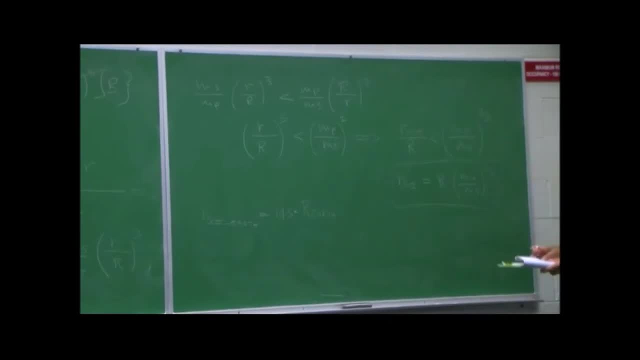 45 times that, Which obviously means can I use? can I say that the moon is outside the sphere influence? Of course not. It wouldn't make any sense. The moon is orbiting the Earth. It better be inside the sphere influence. 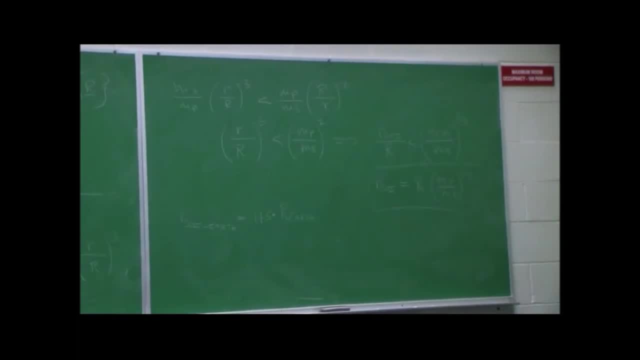 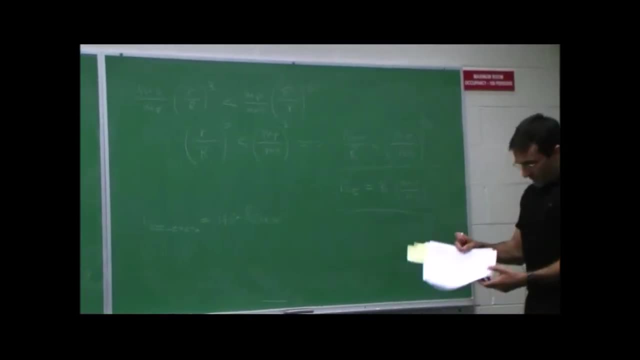 So definitely doesn't apply this approximation to the moon. So if we're flying to the moon, we can't do this patch conics business. You definitely cannot do that. I have a few more numbers, Oh, just to put it in perspective.